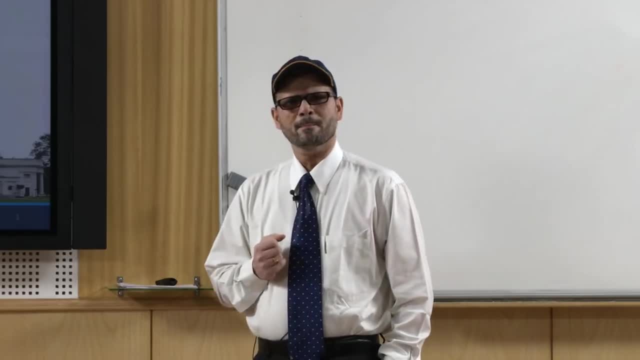 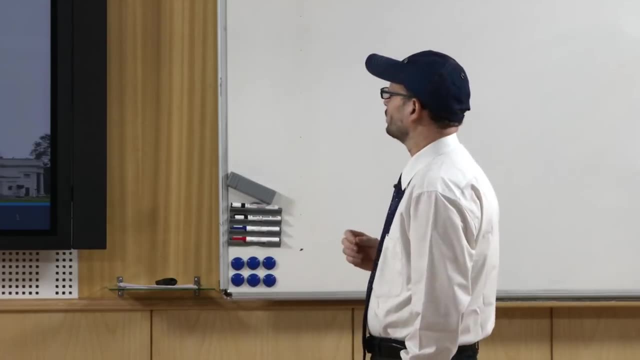 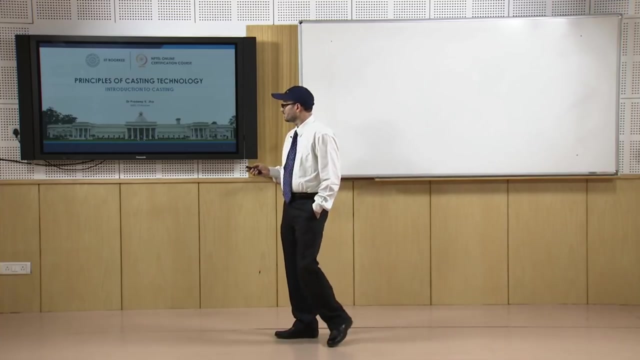 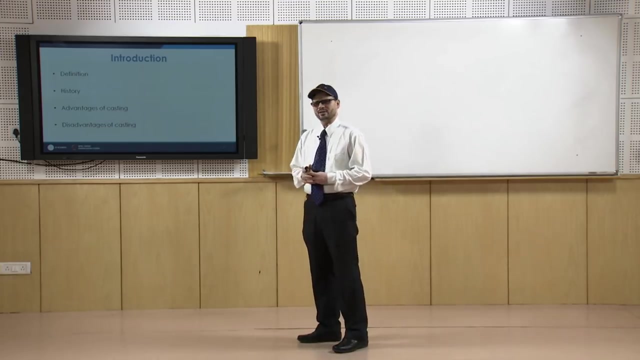 is pattern making, mold making, core making, melting, pouring, finishing, fettling and heat treatment, all that. So let us proceed to the introductory lecture about principles of casting technology. Let us see what is casting. So in a very rude. 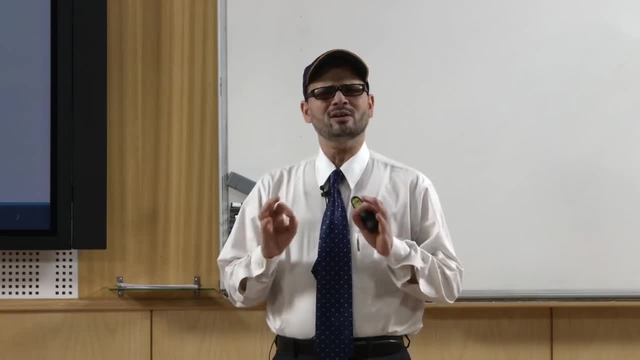 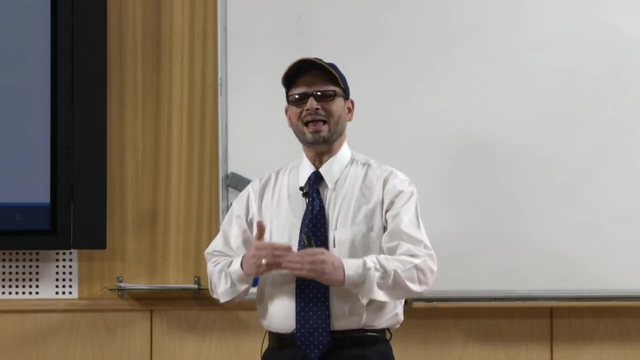 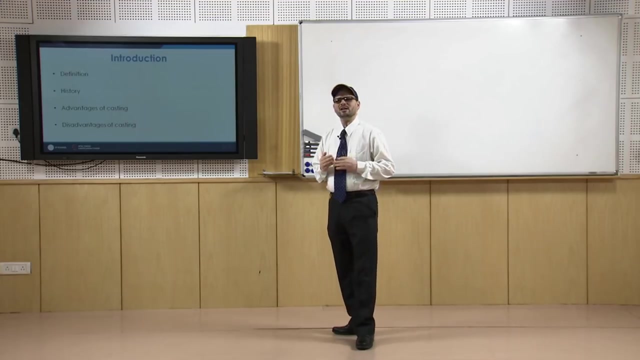 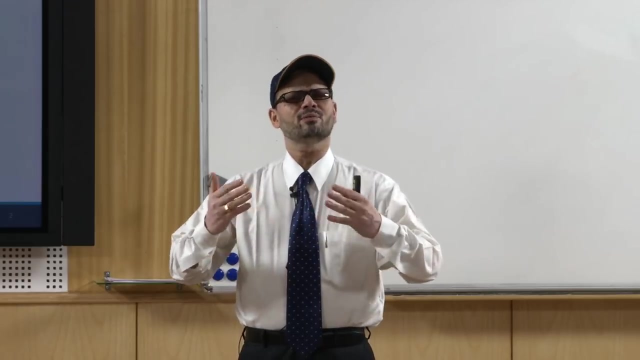 way. So casting is nothing but allowing molten metal to solidify in a closed cavity, or even it be open. The molten metal has to be poured and it will solidify. Now why we need to study this. As you know, the metals have to be saved in different forms. Metals cannot. 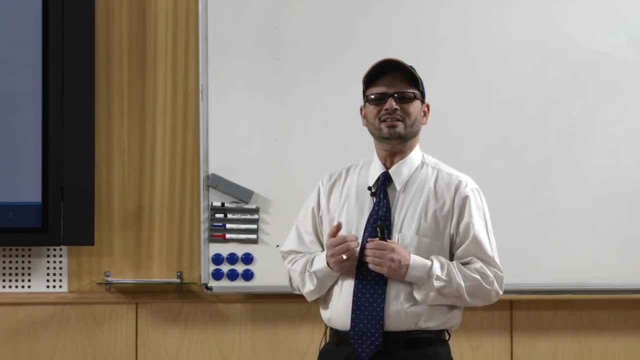 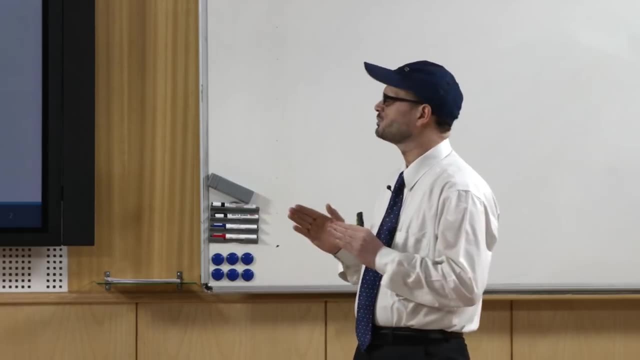 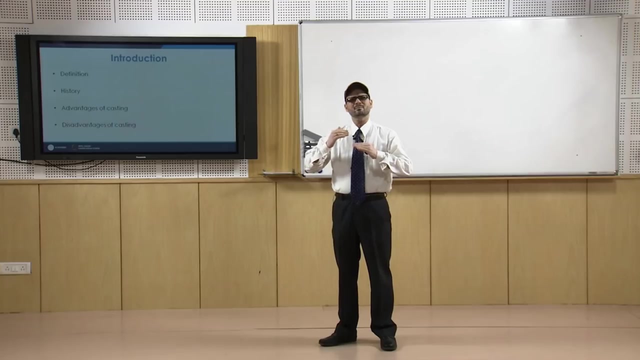 be saved at room temperature. So for all metal we need to make sure that they are solid. So we will use metal to form a solid metal. The liquid state of a metal is called the solid state. For a solid metal it has a lot of strength and because of the solid state it cannot be saved into the shape. 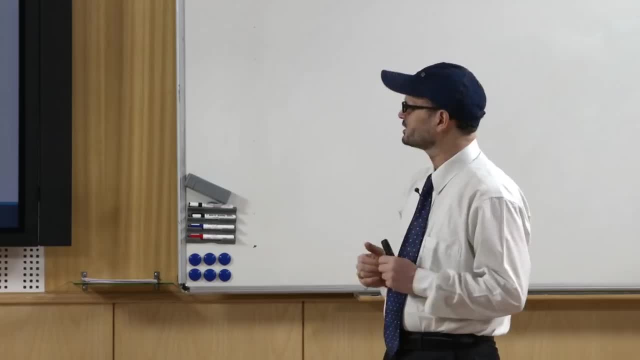 we want. So basically we will have to bring that metal to a state where we can save them. So for that we are taking this metal to a temperature where it is in liquid state, So we are melting it. Then, after we are taking it to another liquid state, we take a solid metal and we 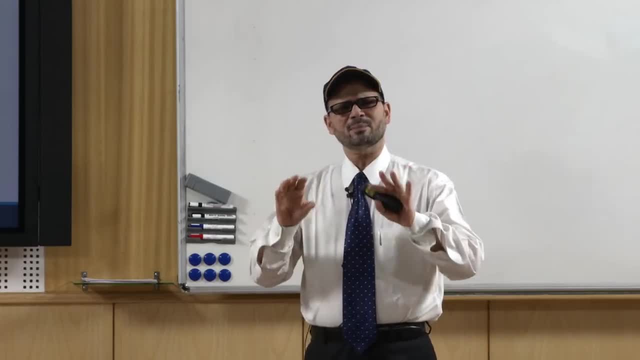 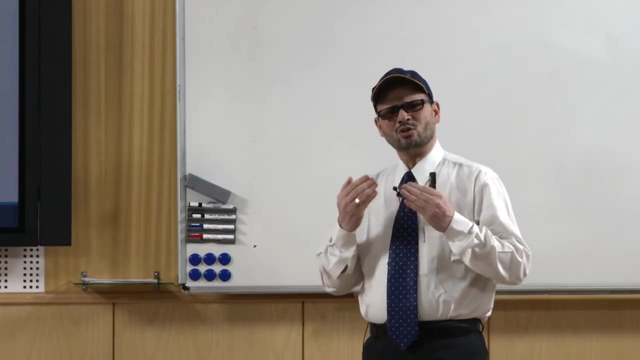 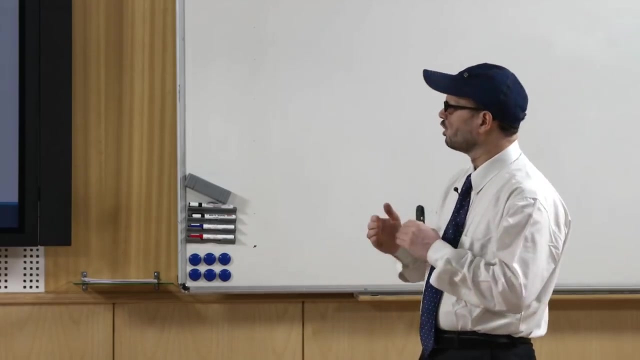 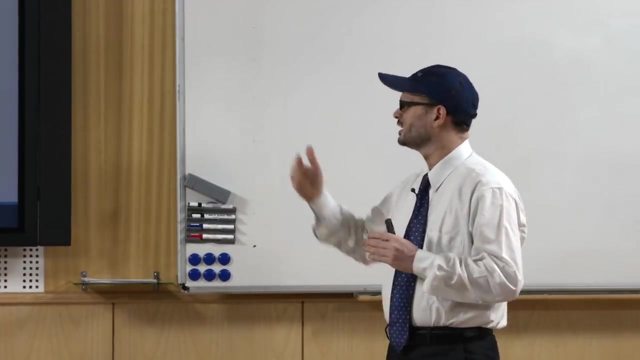 Then, after melting, we are basically keeping it in a cavity. that cavity is known as mold, Now the energy which has gone inside the metal to melt it. this energy has to come out So slowly. once it is in the mold and the metal is subjected to the atmosphere, it loses the. 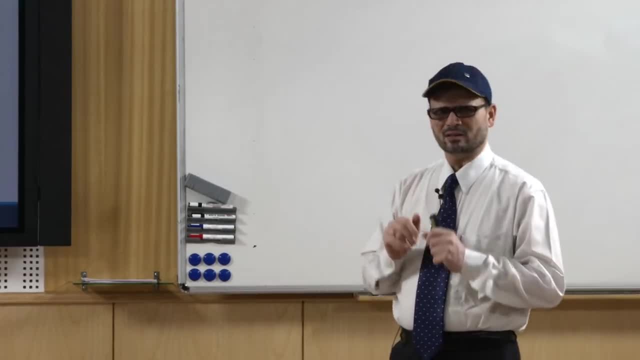 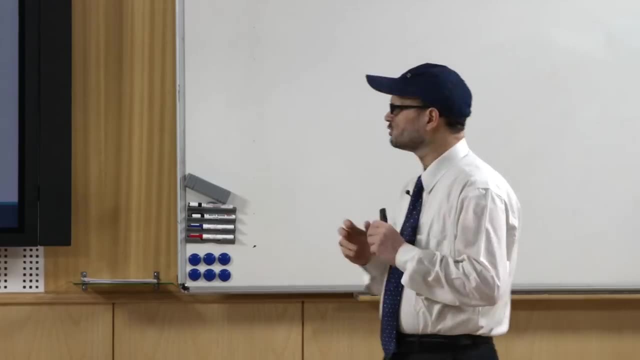 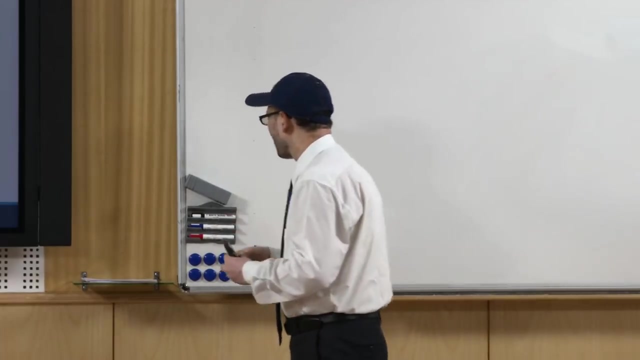 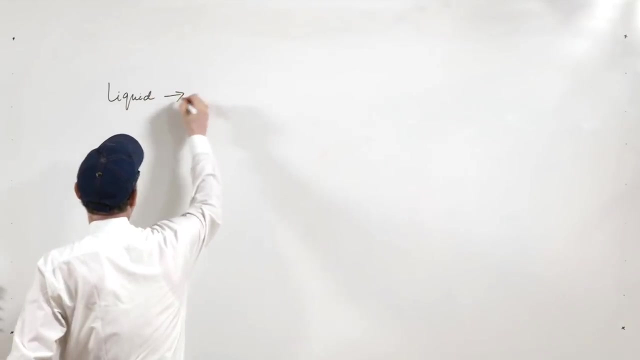 heat which was put in the metal, then it takes the shape of the cavity in which it was poured. So this way, after removing that mold, we get the cast metal. So what we see is normally we see that a liquid, a liquid can have, can possess any shape. 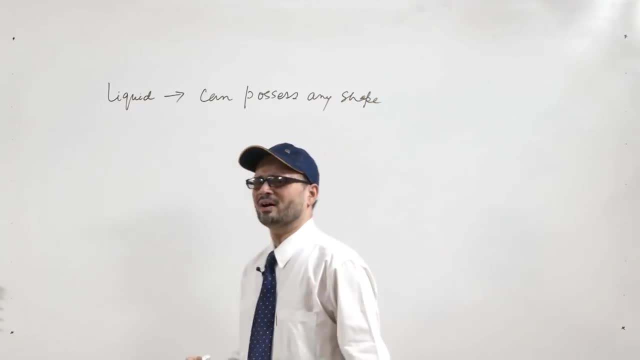 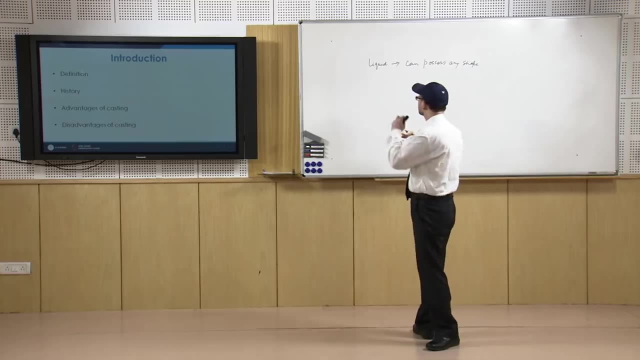 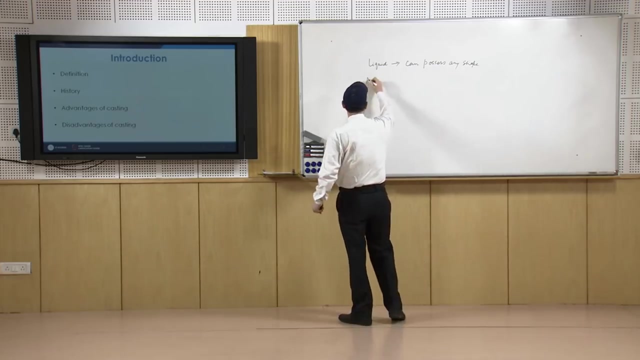 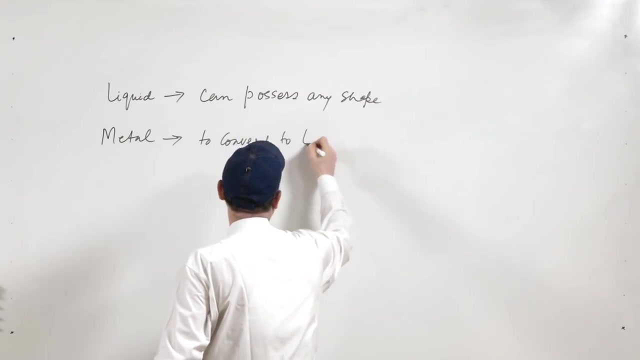 However, for giving the metal to certain shape, you will have to bring that flowability into the metal or it has to have the fluidity. So for metal you have to convert it, to convert to liquid state, And most of the metals have the fluidity. 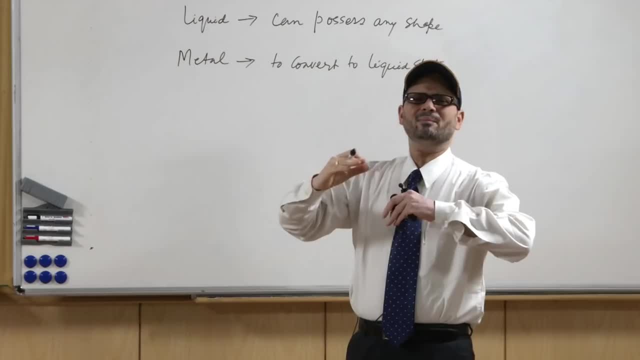 So for metal you have to convert it, to convert to liquid state, And most of the metals have the fluidity And most of the metals have their melting points above the normal temperature. So basically, you will have to give the heat to melt it. 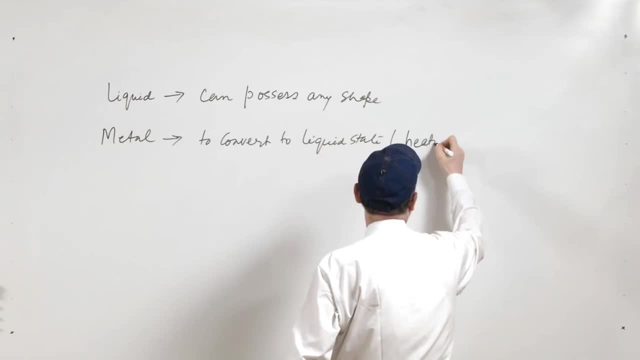 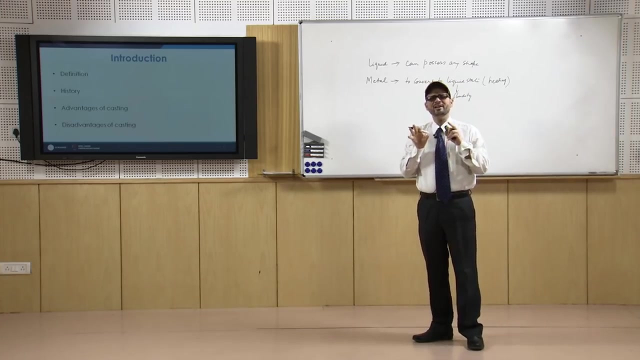 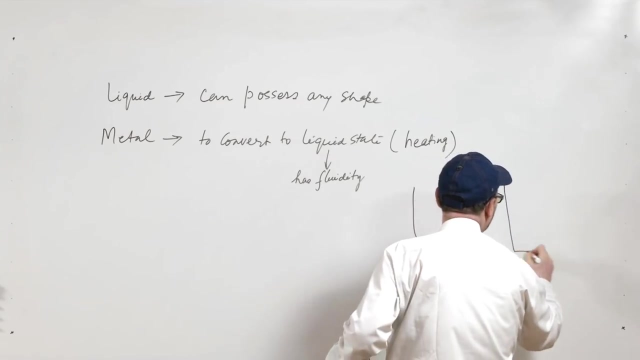 So this can be done by heating. So once you heat the metal it converts to liquid state. This liquid state has fluidity. Now it has the characteristic to flow in any contour. So then you can pour liquid, You can pour in any shape. 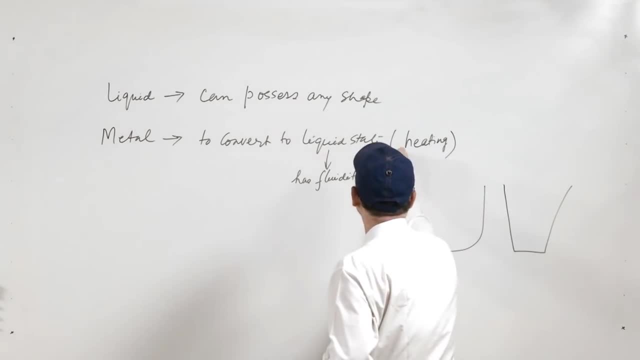 In any shape you can pour this. So this liquid, this can be poured either here or this can be poured in any shape. Once this liquid goes in any cavity and you stop heating, this liquid has to lose the heat, So heat is lost to surroundings. 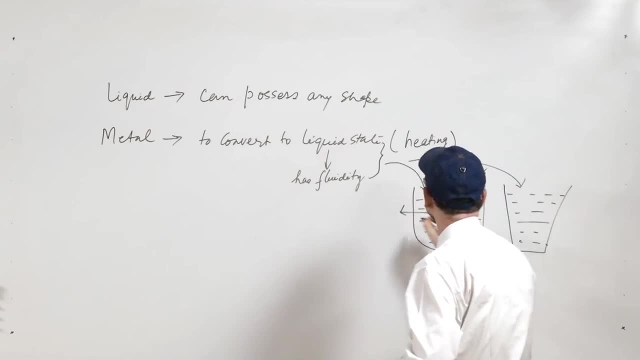 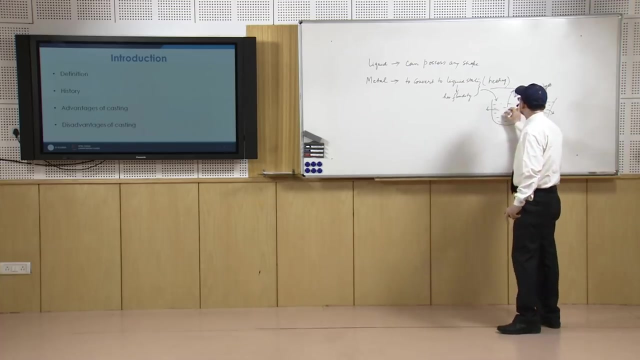 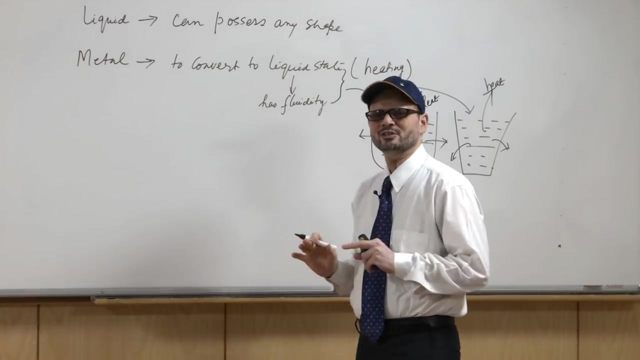 So heat is lost to surroundings. So heat is lost to surroundings, Heat is lost to surroundings, So, similarly, heat will be lost to surroundings After losing the heat to the surroundings. basically, a state comes when it is coming at its melting temperature, So that is known as an equilibrium temperature, below which the metal will be solidified and 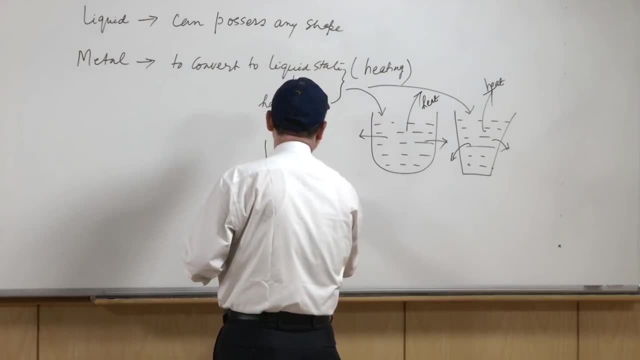 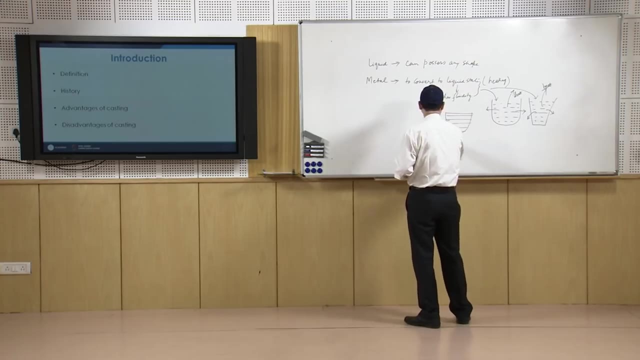 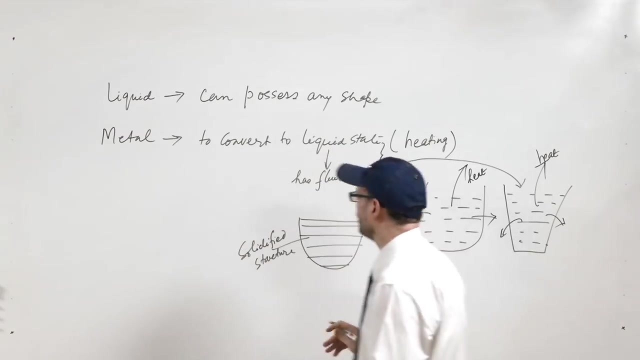 it will come in a solid state, So it will be a solidified structure. So basically, once this liquid has lost all the heat and it has come to a temperature lower than its melting point, then it has come to a solidified structure. This shape can be a complex structure. 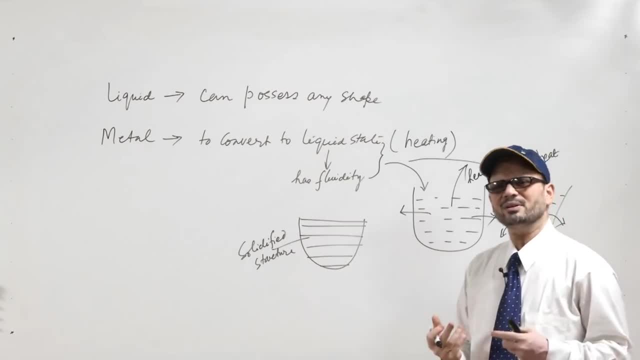 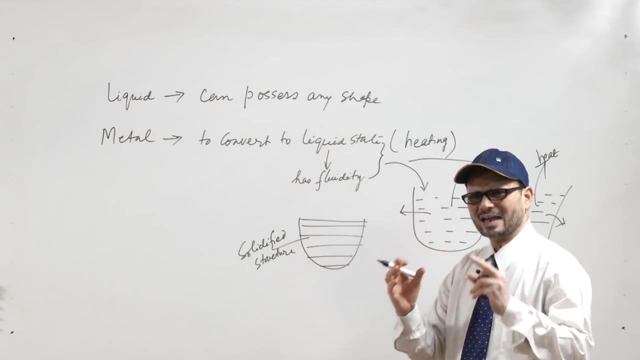 This shape can be a complex structure. This shape can be a complex structure. It can be a simple shape. It can be a simple shape. You may have to go for a number of changes to get the type of shape you want. So this is how we go for casting. 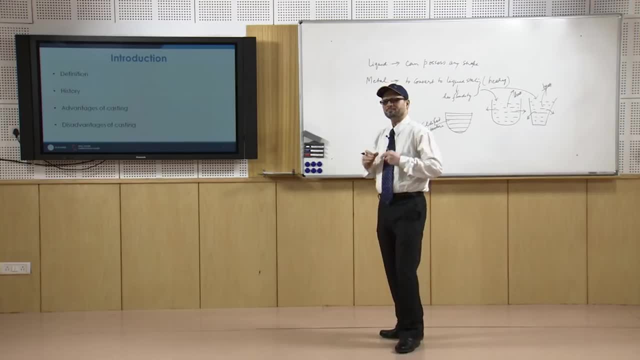 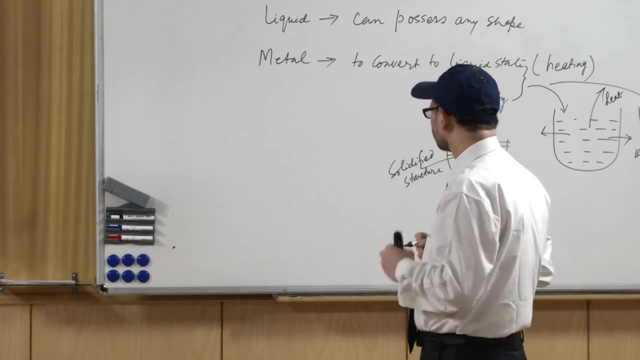 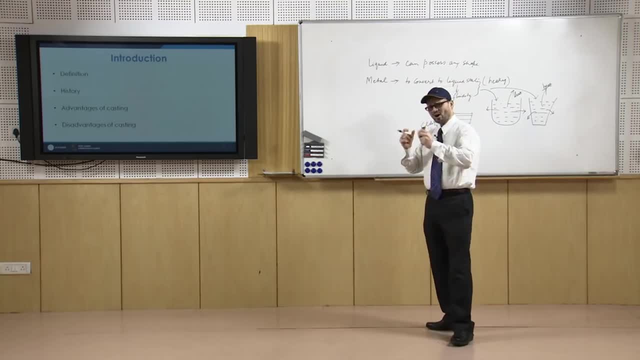 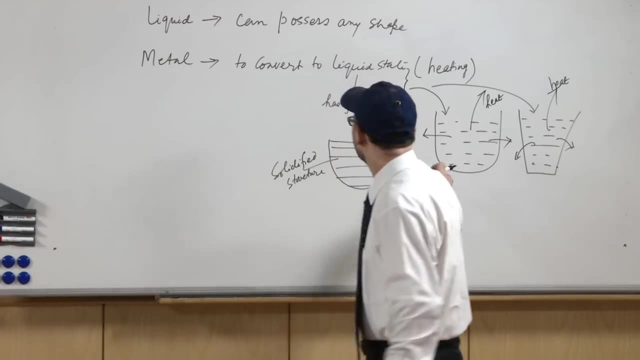 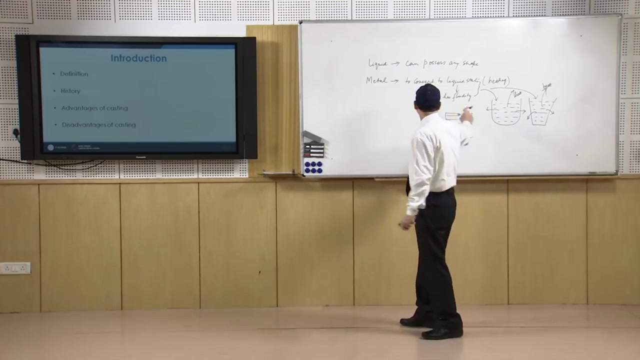 5,000 BC, So even the ornaments. they were made and they. it has been reported in the civilization earlier civilization that this process was there In the earlier days. basically, the mold was made of either sand or even stone, So earlier stones were used, it was carved, some portion of the stone was taken out and 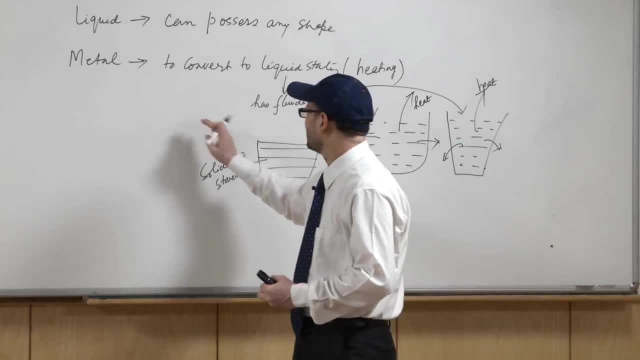 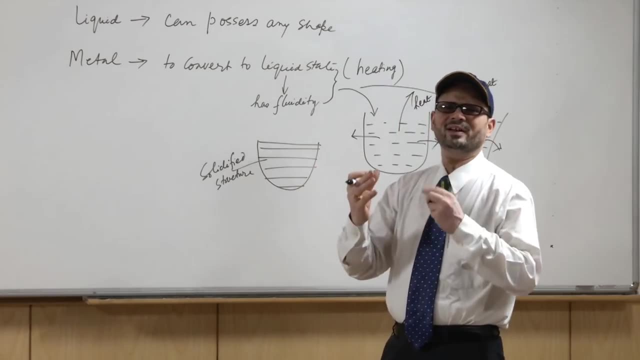 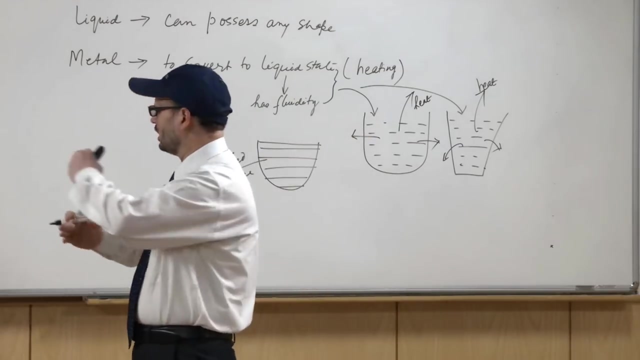 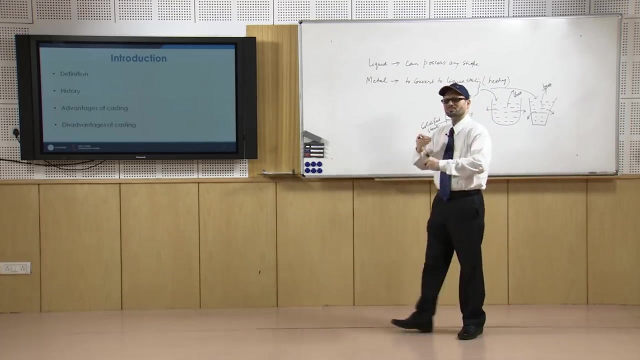 in that portion you were using the metal, liquid metal, and so that it gets cast, and taking the stone parts out, we were getting the different types of metal and those metals were in the form of, you know, tools used for killing the animals or maybe for the agriculture purposes. 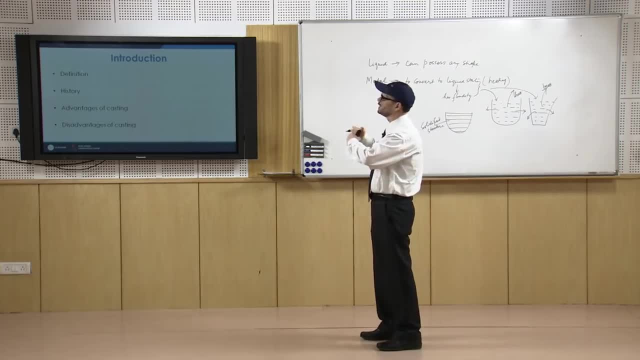 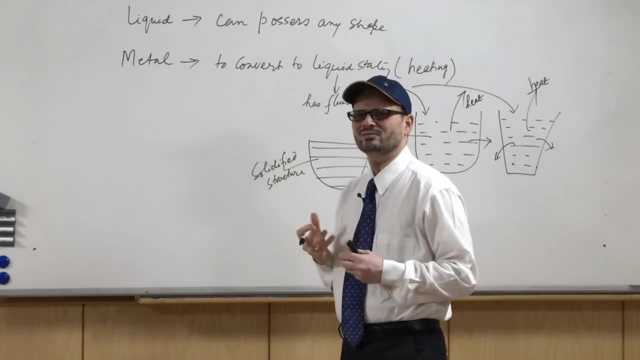 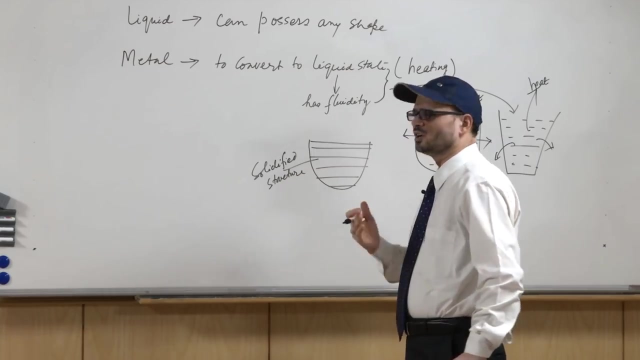 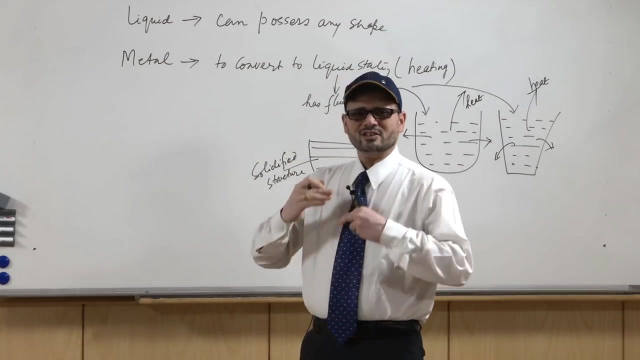 these are reported in the history So we can have This information about the history. how chronologically this casting process has evolved, that is another matter. but we must know that this is the process which was there in our earlier times and even in the modern days still advancements are going on to see that you get a good structure. 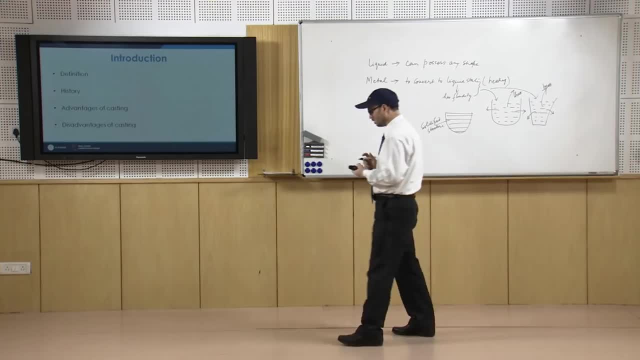 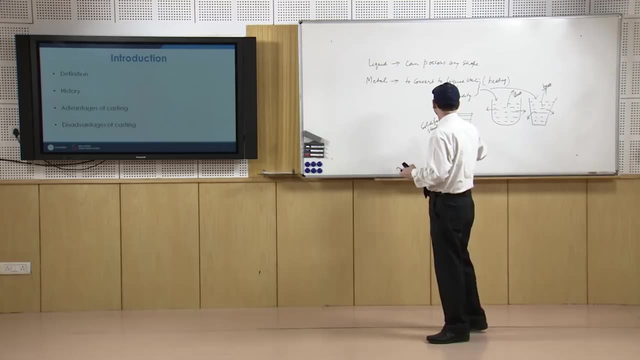 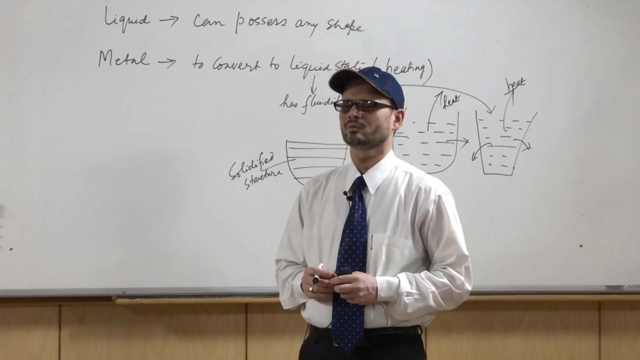 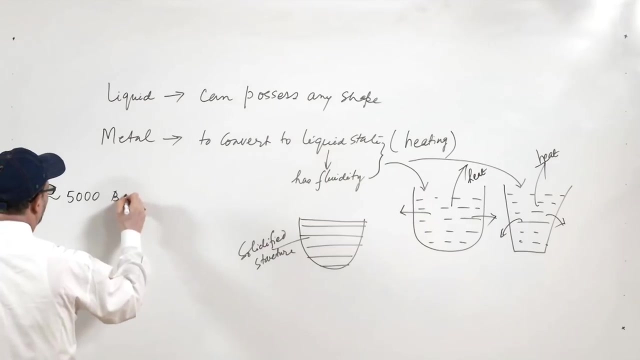 and good property of the cast metals. So if you look at the history of this casting process, we should look at certain milestones which are considered as milestones in this field. So in around 5000 BC, the, it has been reported that use of knives 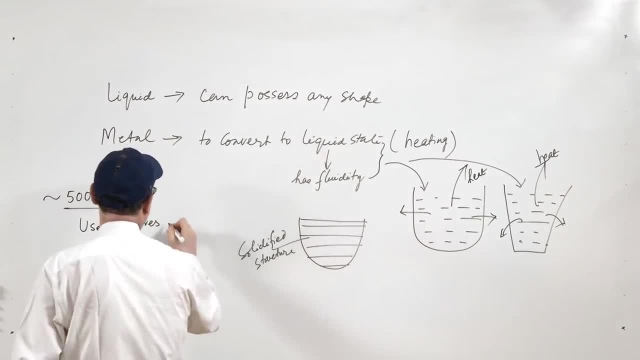 Now ca nutritions ingest, the used希ords can gdyn and all these fuctions are repeated in largevity when we move over the land section and systems collapse. So if we are talking about the history of this casting process, we can see there were 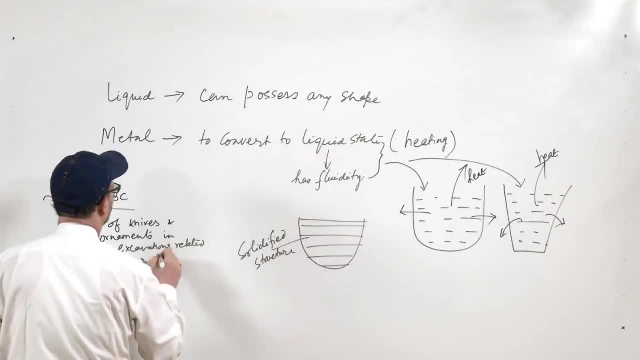 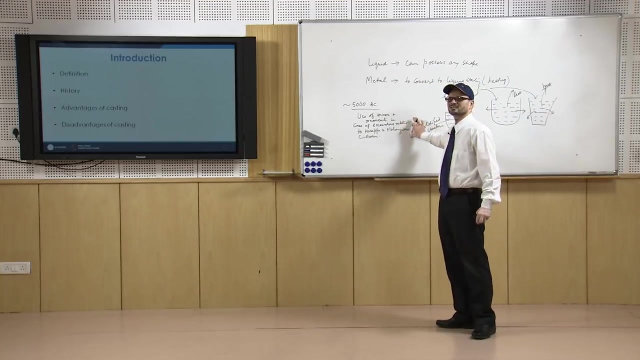 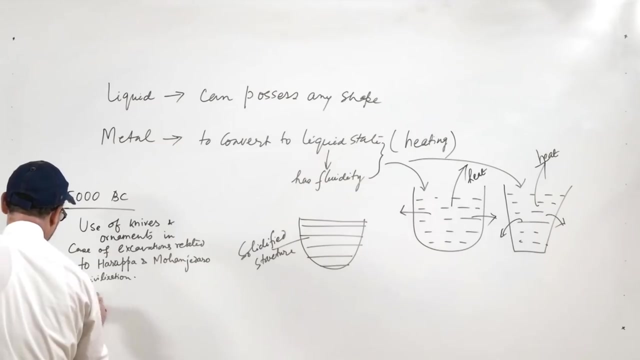 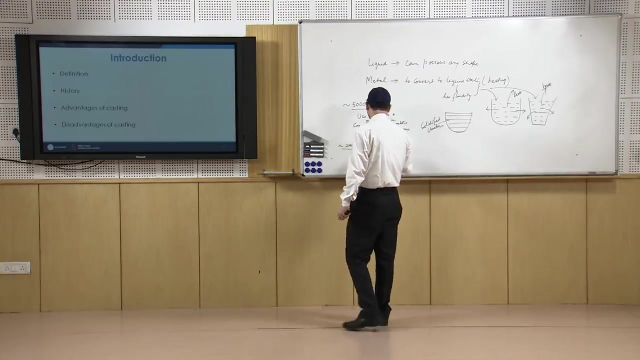 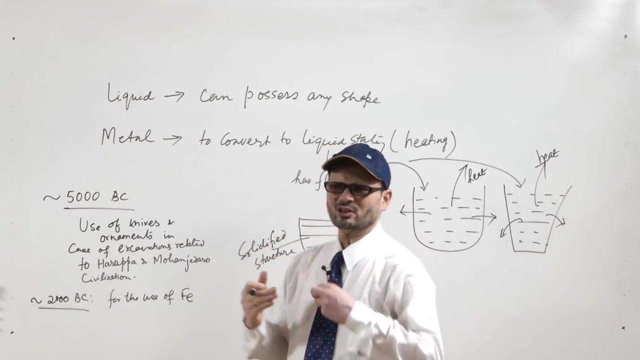 3 milestones. So in those days also it has been seen that this was there in its place. around 2000 BC, first time the Greeks were supposed to be the users for the use of iron. These applications of this process was for the guns, for the tools. 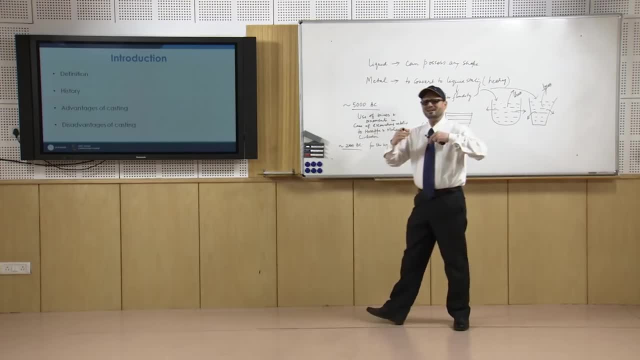 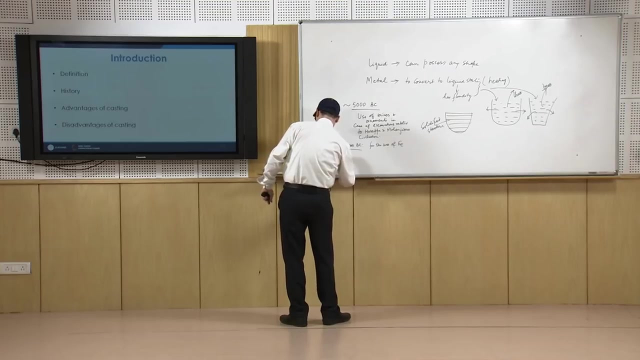 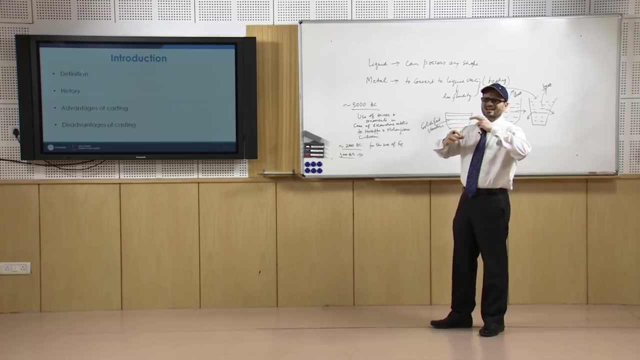 In case of other metals. you know, earlier the copper and bronze was mostly used for making either utensils or the tools, The statues, monuments, all that were used, I mean the most. mostly it was copper or bronze. Now, in the 500 BC, there were also. there was something like a revolution in the case of 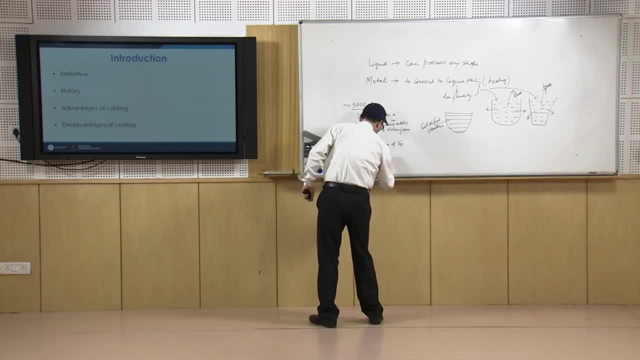 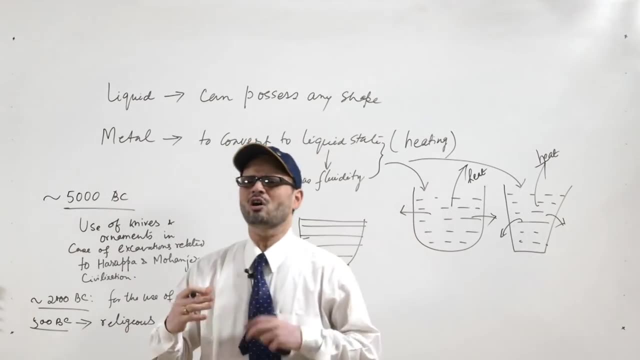 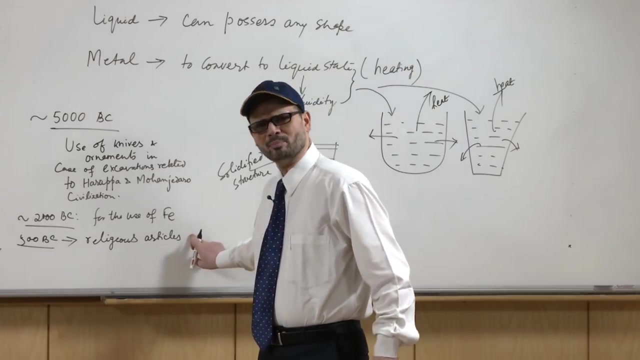 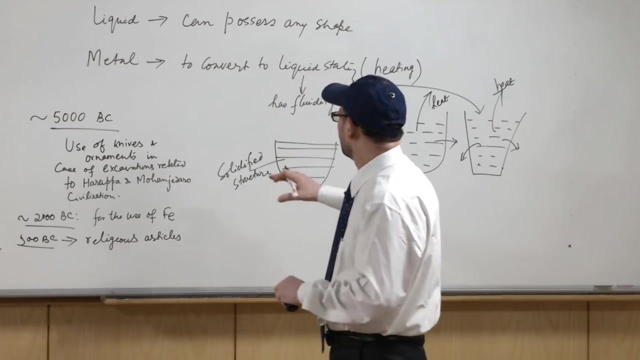 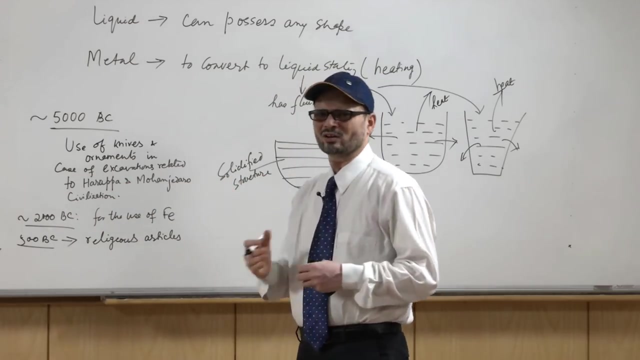 religious art Articles, like the statues of gods and goddesses. they have also been reported and it gained a lot of momentum. So this is how the history, in a very nutshell way, we can say that it has come since long and still it is going on. coming to the 19th century and 18th century, there has been a 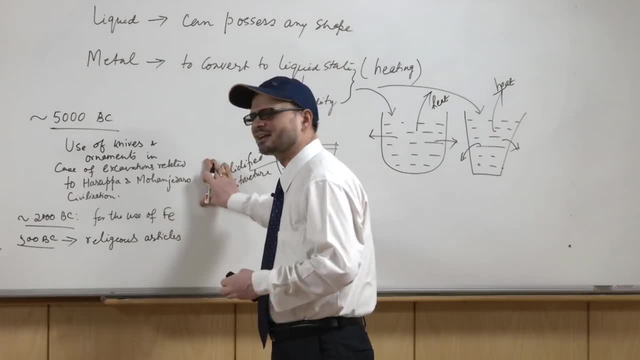 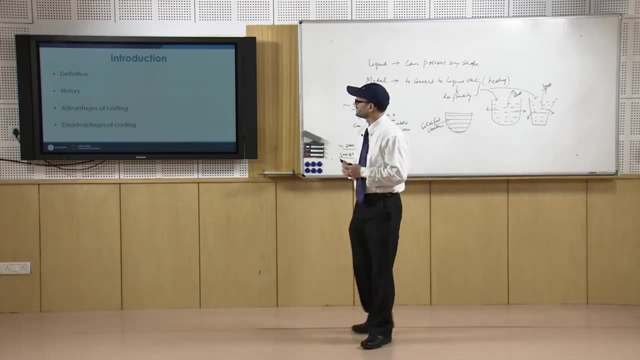 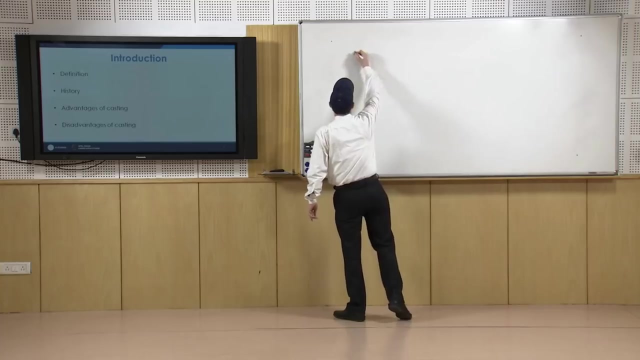 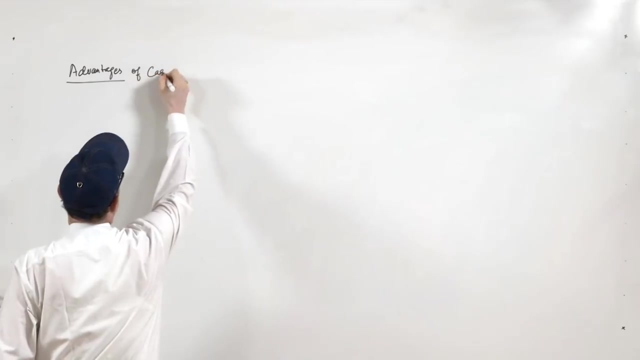 lot of improvement, And that can be found out by going into the history of the casting processes. Now we will discuss about the advantages and disadvantages of casting. So first we will discuss about the advantages of casting process. 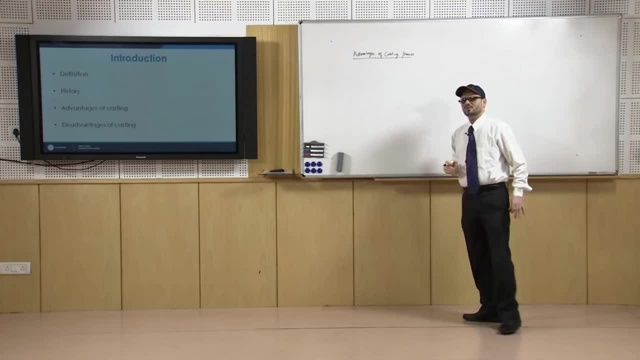 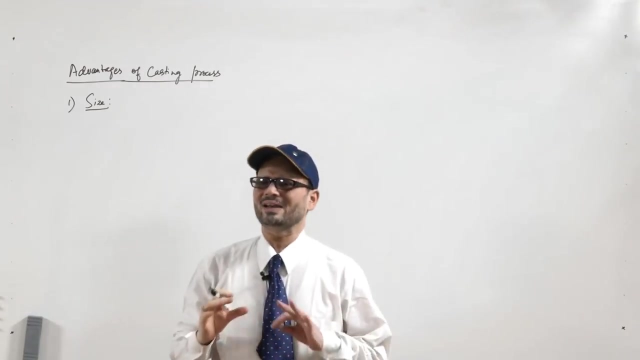 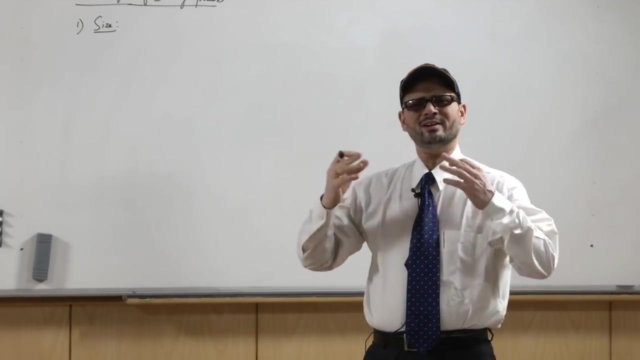 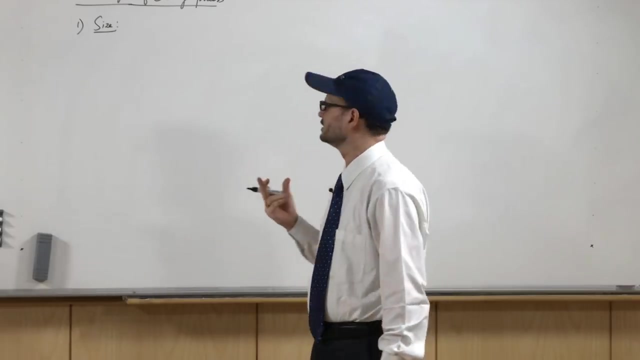 lot of advantages of casting process and we will discuss it one by one. first of all, the size. you have the flexibility to cast a metal of even up to 200 tons or even more, and you may come down to even a wire of 0.5 mm diameter. so size is a very important factor when we 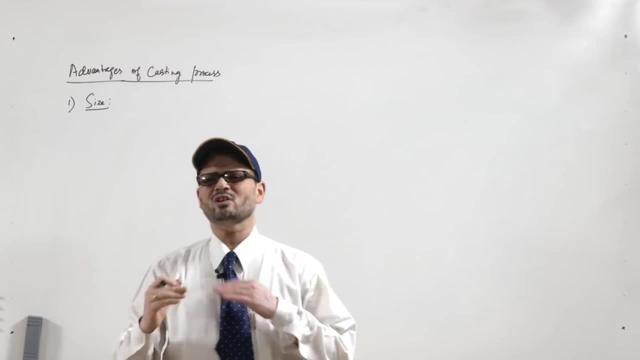 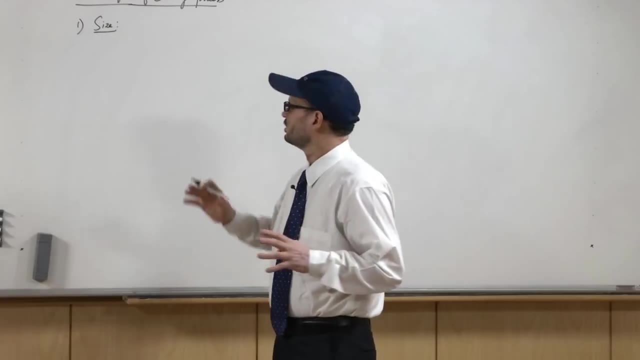 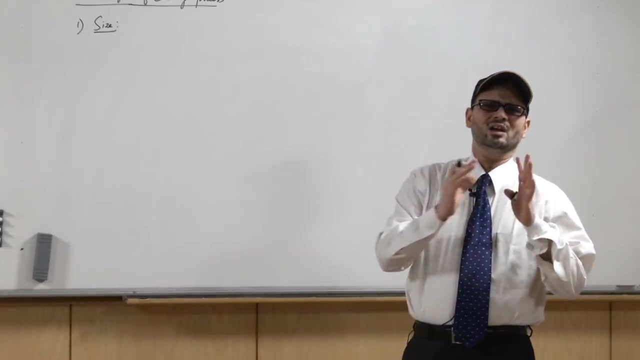 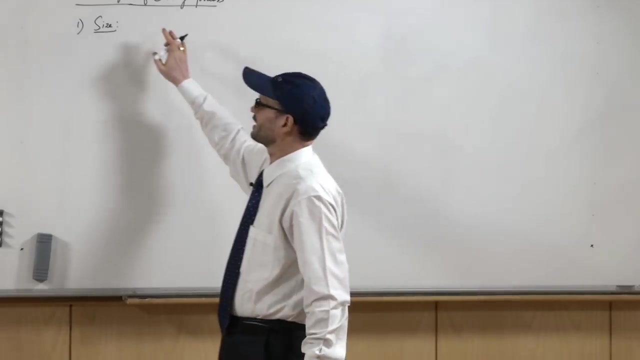 talk about the casting process, specially when we talk about the larger components, having the component in one go. it is only possible by casting process. otherwise you may have to assemble a lot of other components And then you have to fabricate them, you have to join them. so this is a great advantage. 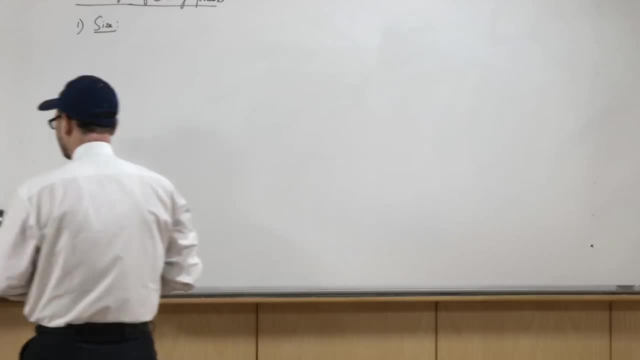 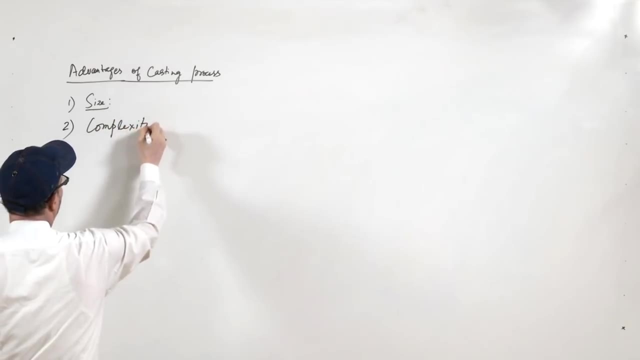 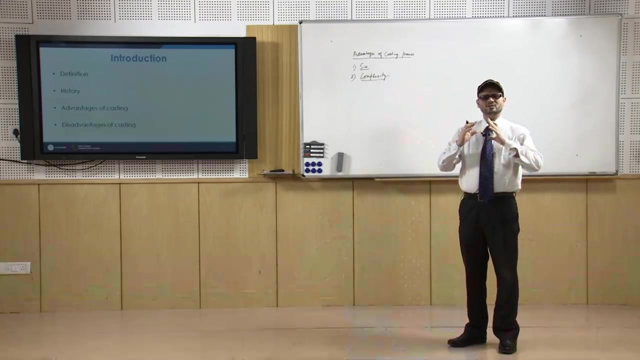 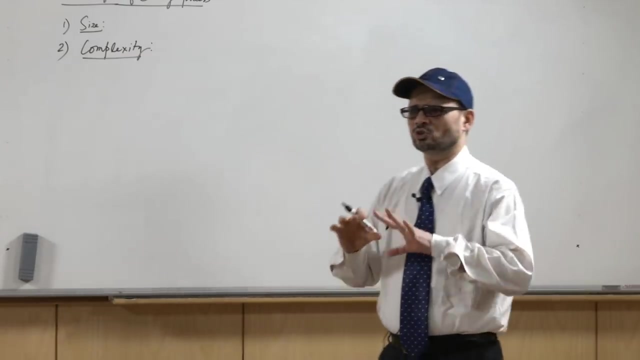 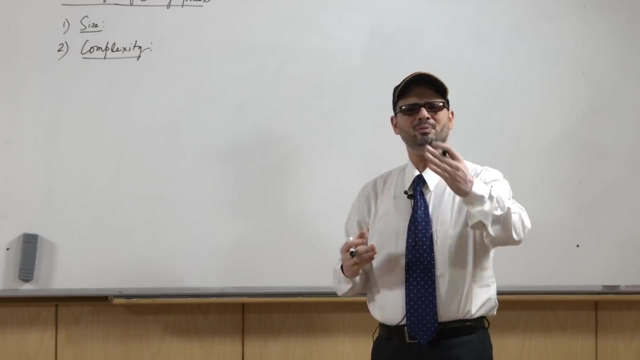 in case of casting. Next is complexity. you can cast a metal of very simple shape to a metal of complex shape, either externally or externally, So you can have a mold of that particular shape and, without the need of any further operation, you can get the complex shapes even in a single run. 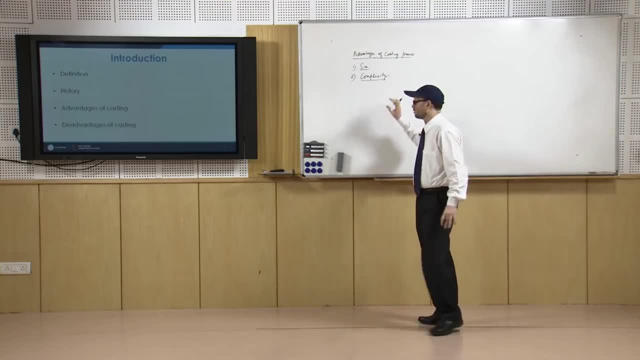 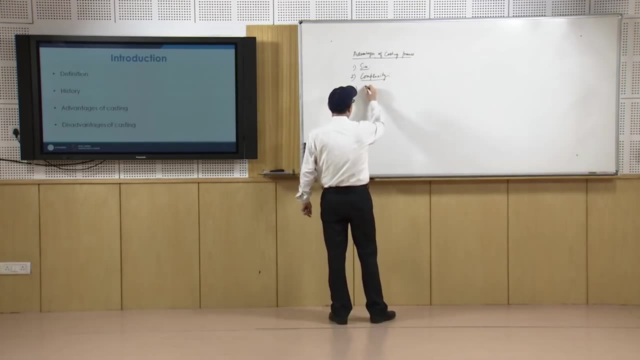 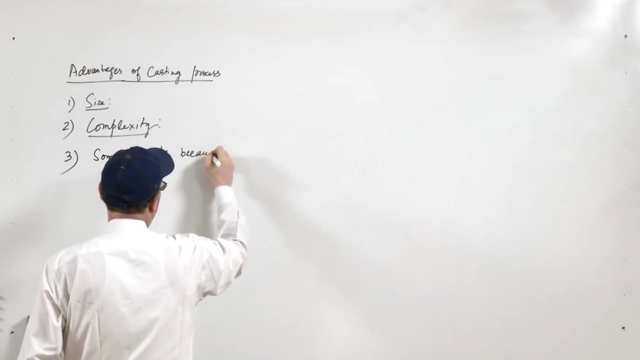 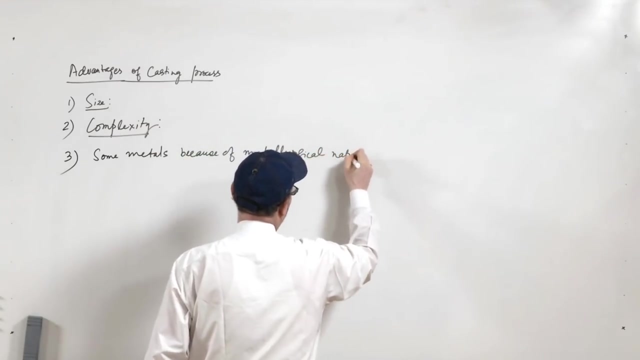 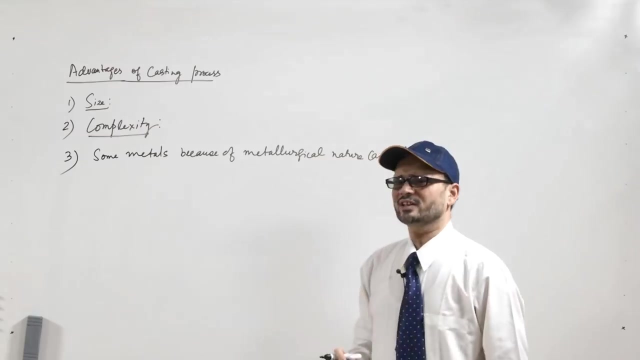 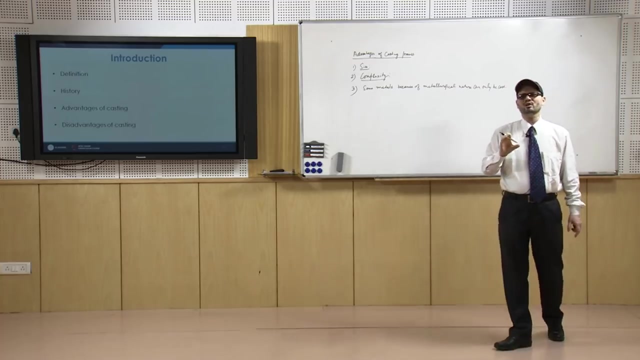 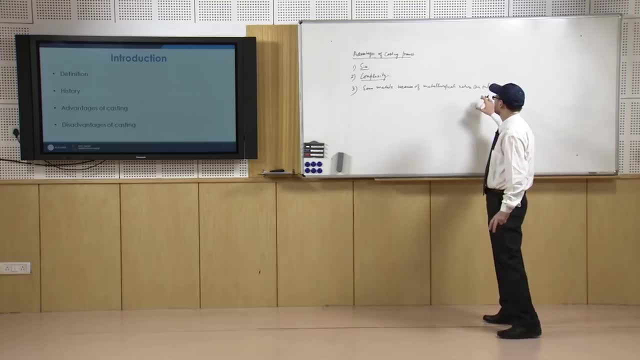 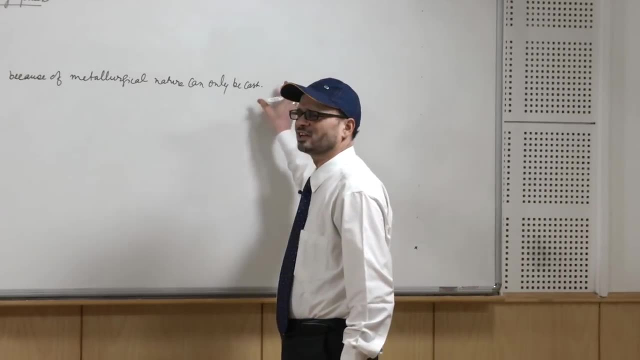 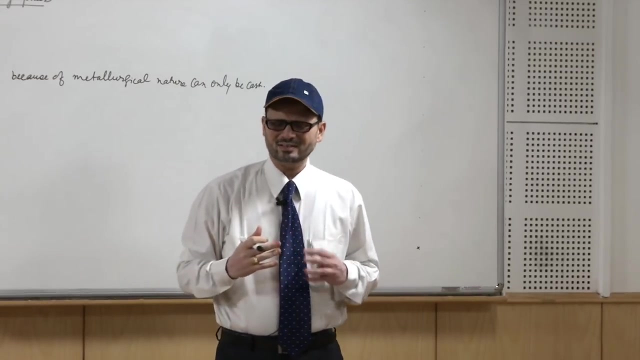 for certain metals because they cannot be formed by other processes, like phenomenon, like forming. The typical example under this case is cast iron. So when you have the metallurgical limitations, like all, we know that in case of cast iron, basically because of the presence of 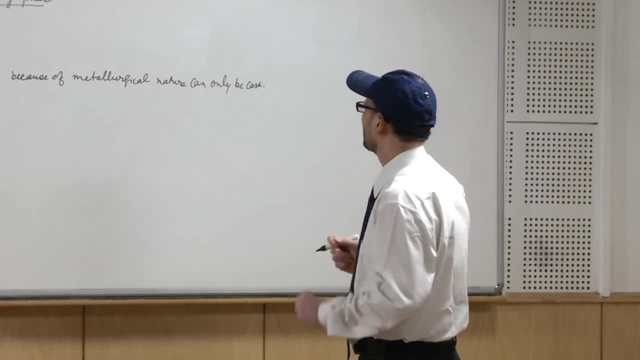 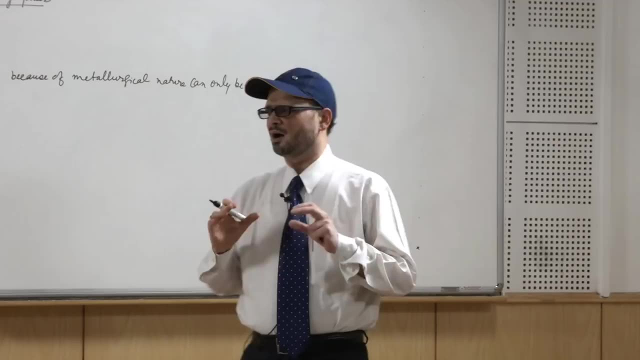 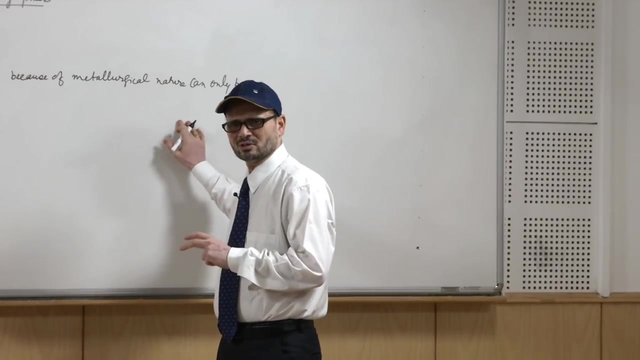 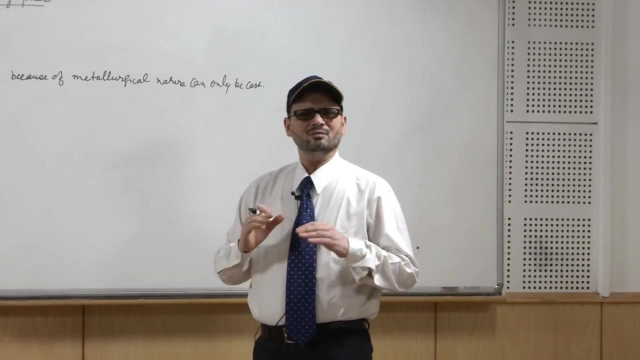 graphite in the form of flakes. it has a very low toughness and it cannot be formed. it cannot be forged. So in that case you have no option but to only cast, and we have in that case only to go for casting, because cast iron, for example, has a lot of advantages. it has a good machining property. 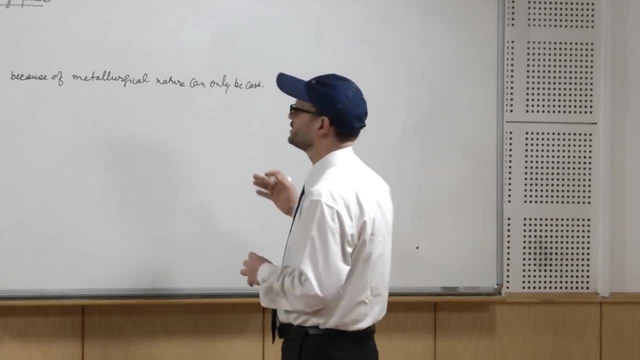 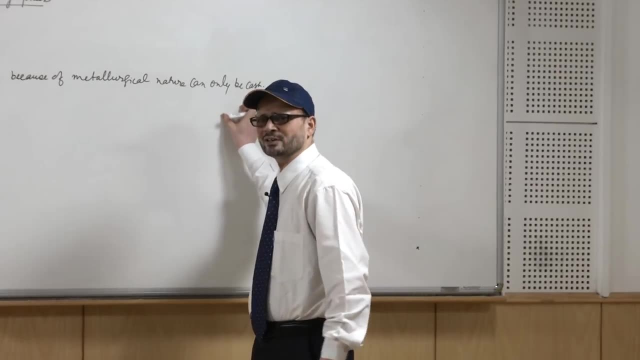 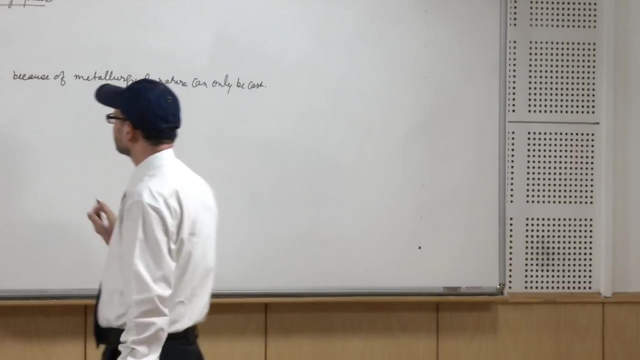 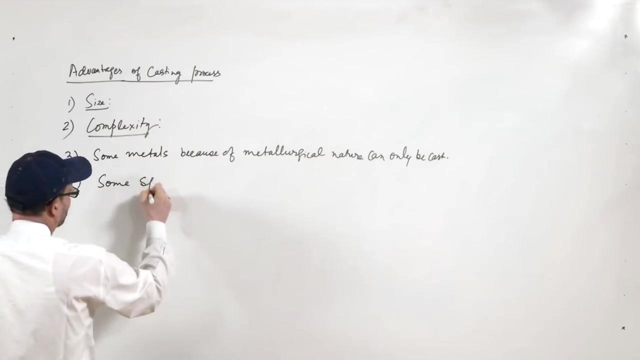 it has a good damping property under the when they are subjected to vibration. So for these benefits you have to only adopt casting. So that is one advantage of casting. Now, some of the special properties are only achieved through casting process. 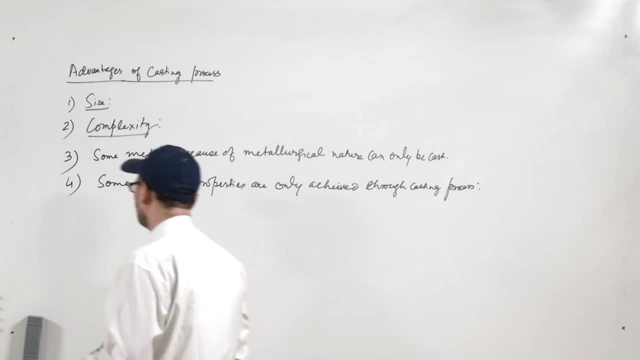 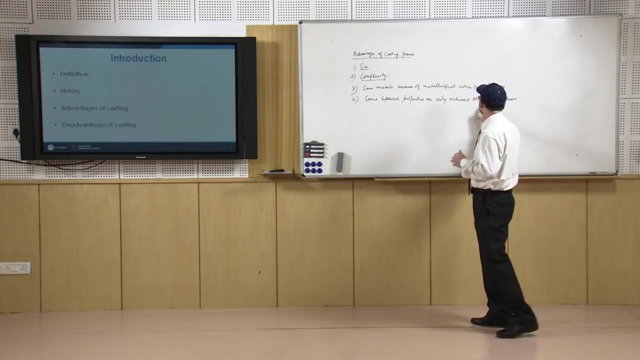 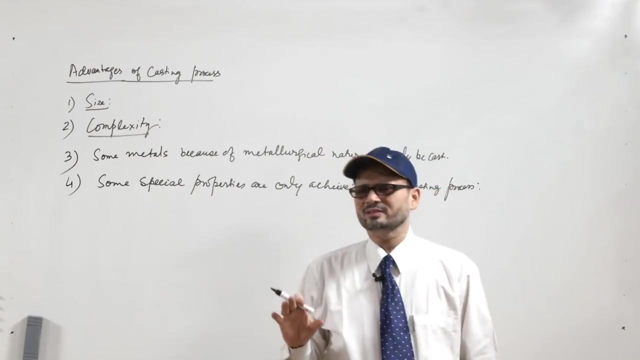 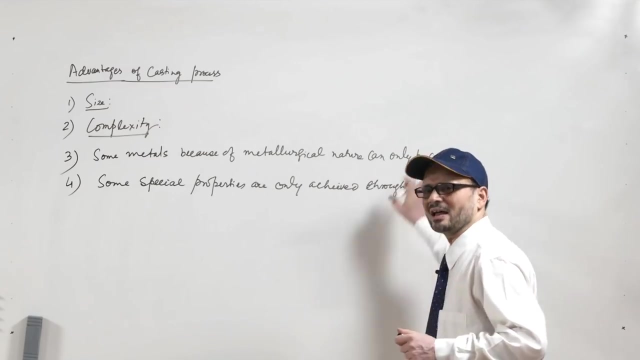 So, basically, when we talk about certain metals, some of the qualities are only achieved when we talk about the casting process only. They cannot be achieved if we are making the product through forging route, like what we discussed about cast iron. The cast iron has good machinability property. 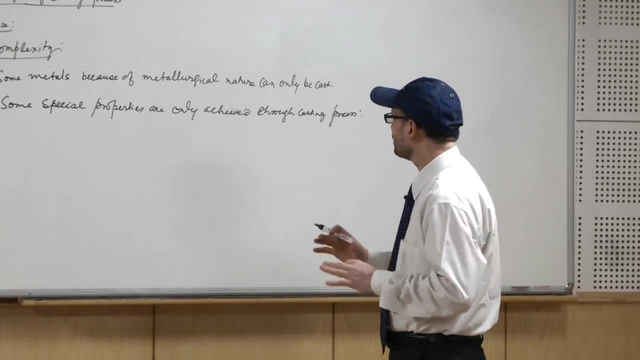 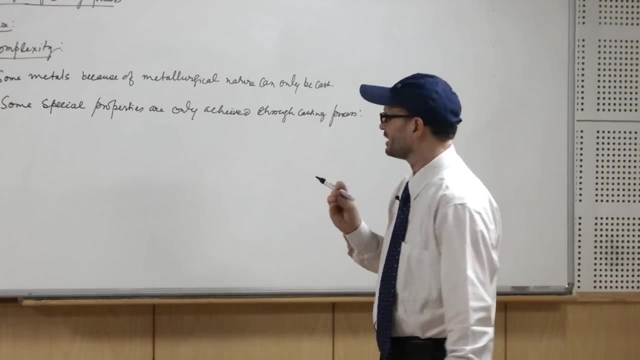 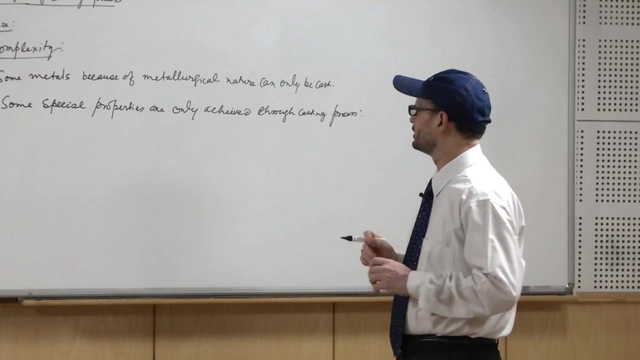 or the good damping property because of the presence of carbon in terms of graphite flakes, which are soft, and that is why it gives a very good machinability, as well as the cushioning effect gives a good damping property. So that is that. Another example is like you have many. 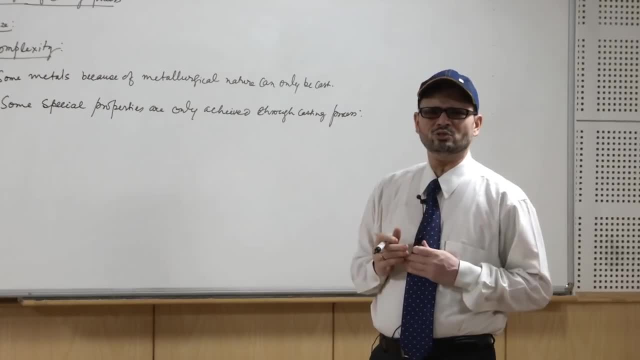 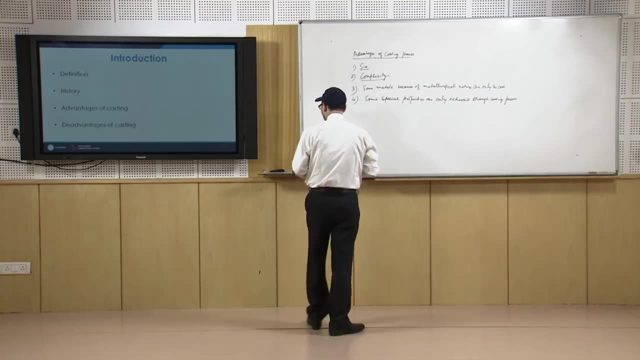 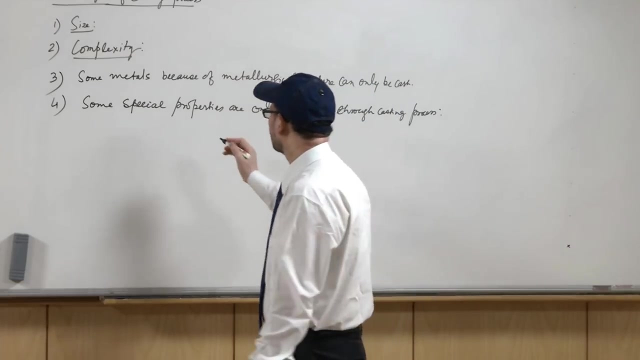 example of bearing metals, So that property is also achieved only in case of casting. So this particular semi certain solution is call Como iron Sure, what we first mean and then we say, because in the same kind of wood there are many iron and this particular be able. 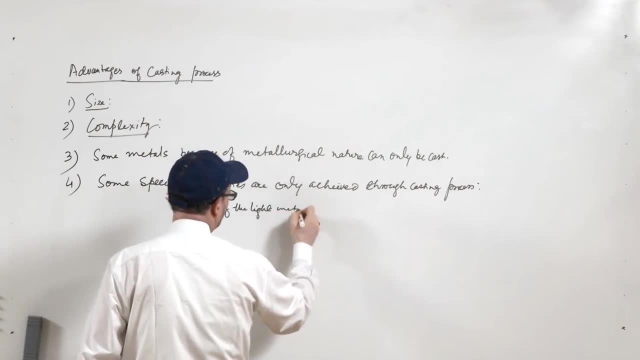 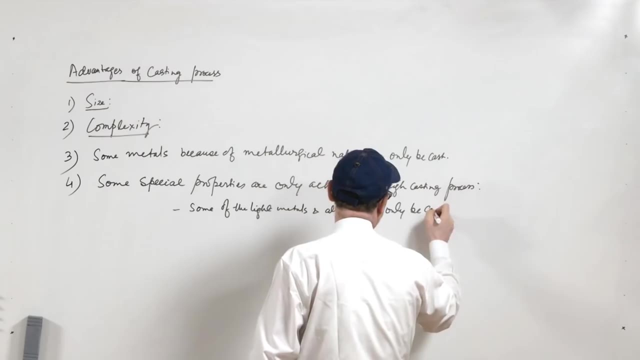 to be made knock. The organic line is not there, годаity. So flat earth material is very thinai. if you have a using in the colluvial structure, It is called a scatterity because it is excels in the nature of a product. so this particular material, they are very expensive. 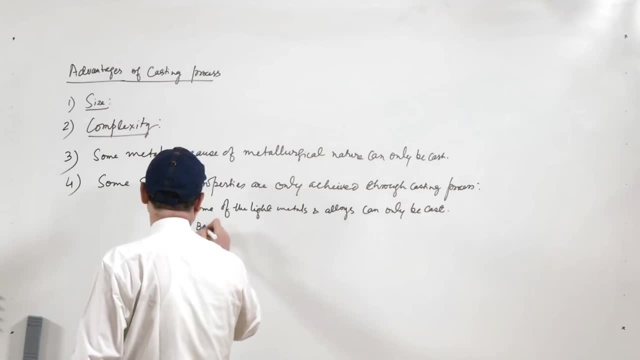 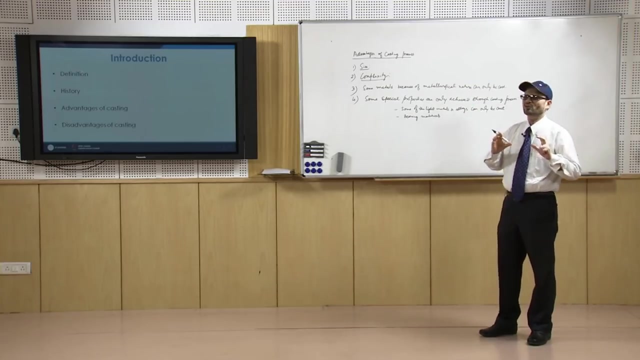 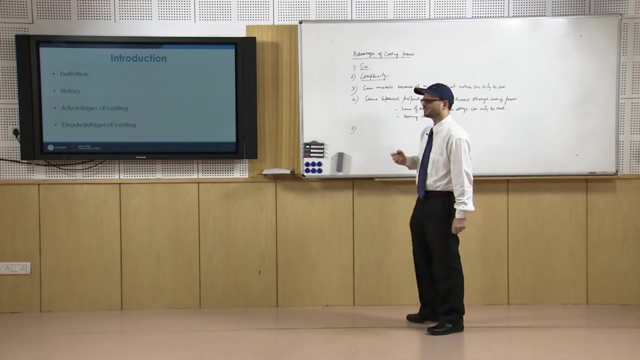 The other Porter is what we look at may be the toughness of the materials, some of the. We also discussed bearing materials, the properties of bearing. that comes only by casting route. when we cast we get the material for that desirable properties. The next advantage is about its cost. 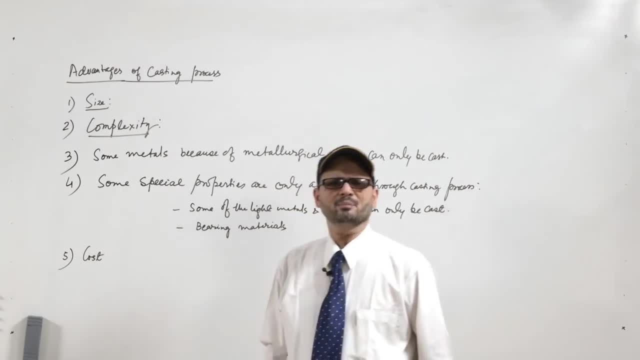 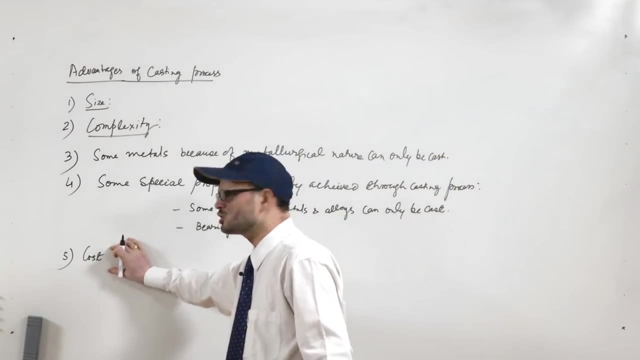 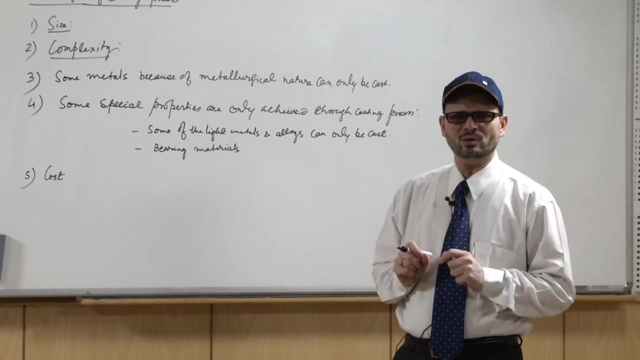 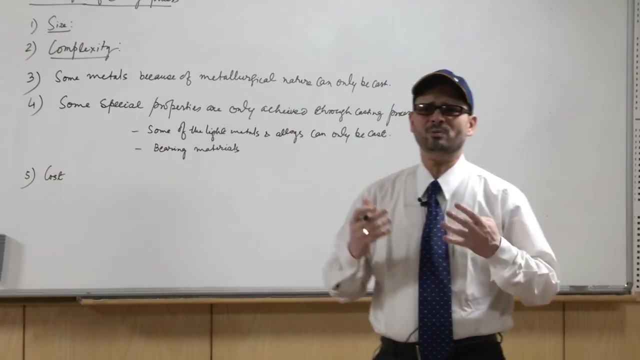 This is the most important aspect because, with respect to other processes, it is economical, as we have understood, that here in one go you are getting the finished product. you are melting and pouring into a mold and taking out and, although it is not completely finished, and you may get even a finished product if we choose suitable melting material. 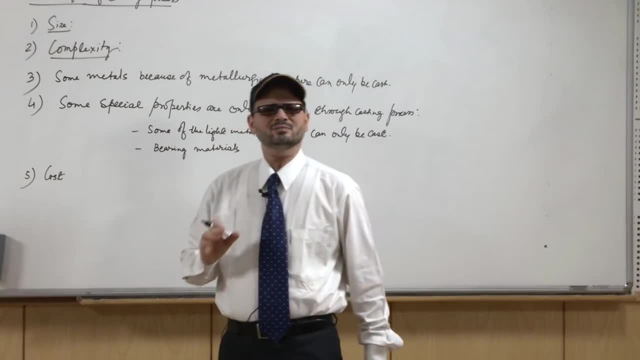 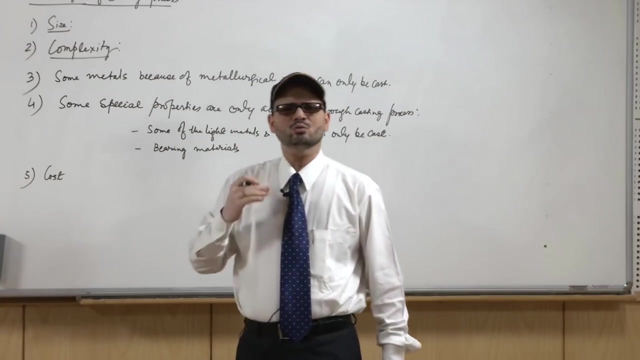 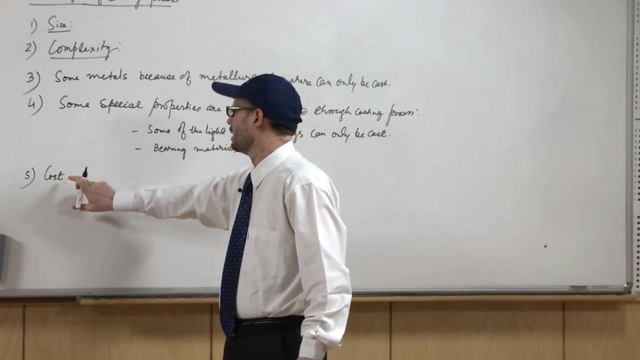 So in that case the cost Of the component. when we talk about making a finished product, the cost through this route is minimum. So when we talk about the mass production, the casting is the only way to go. for if we are getting specialized property, then only we have to think about it, and that time the 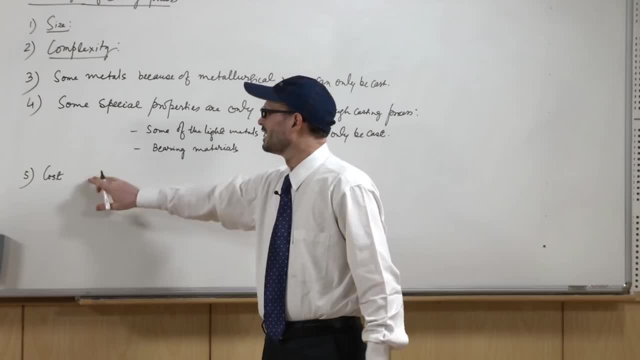 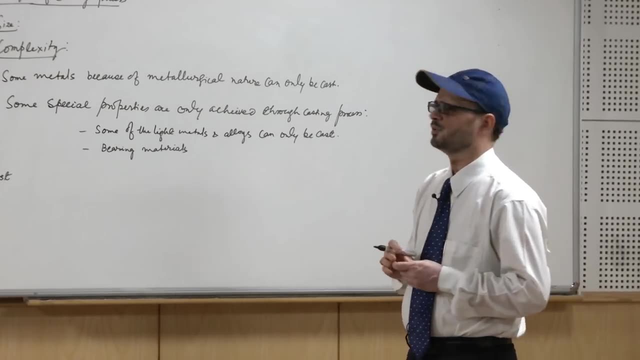 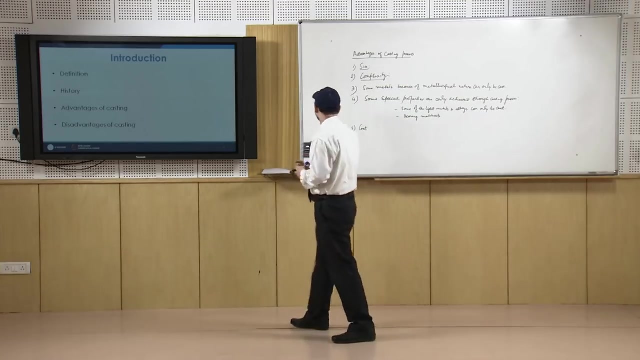 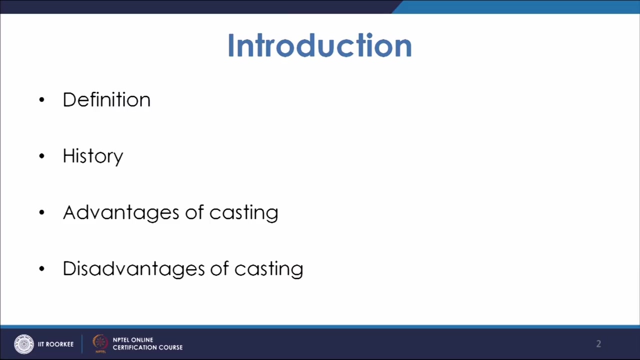 this factor is becomes very important, And that way casting is very important, And that way casting is very important. And that way casting is a preferred process by which we get the material in the desired shape. What is the disadvantage? Let us talk little bit about the disadvantage of casting. 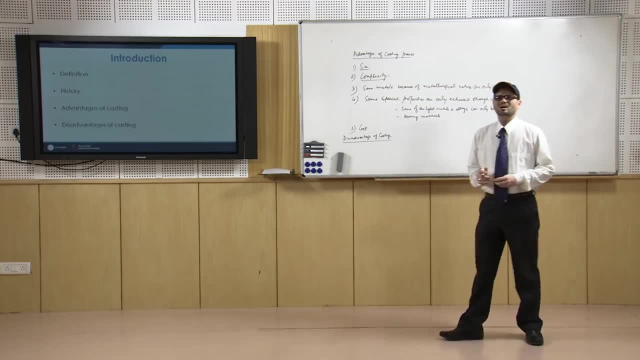 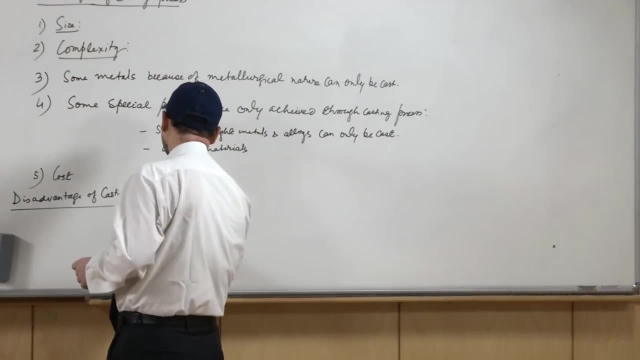 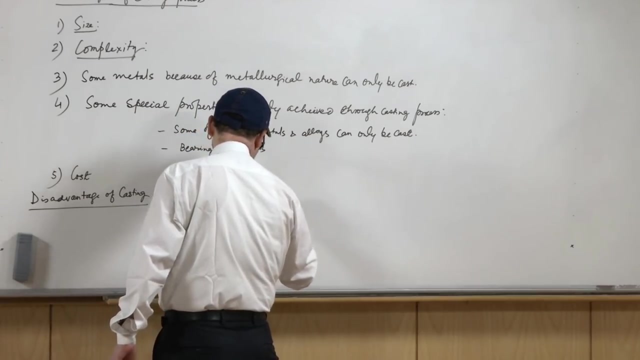 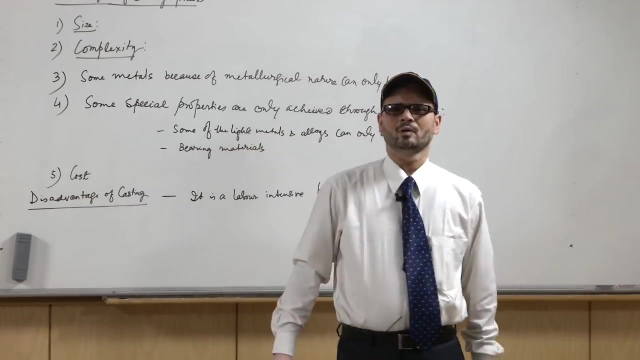 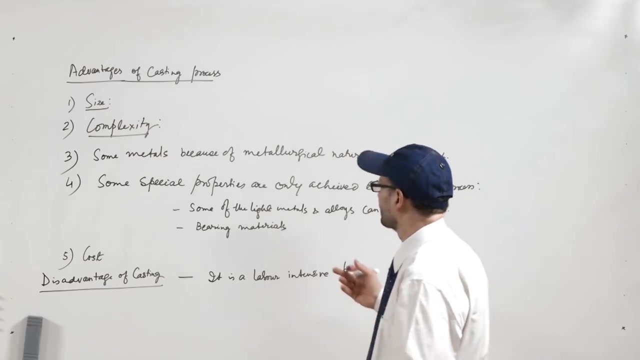 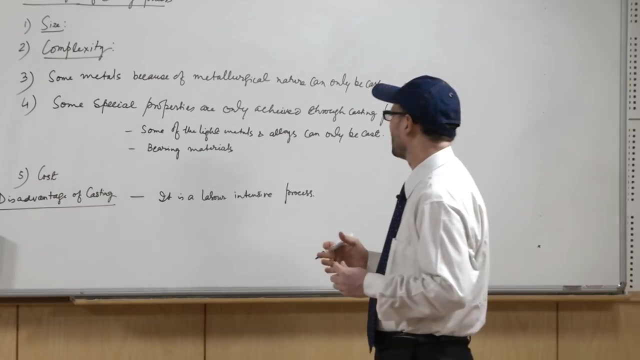 So, although there is not much of the disadvantage, but some of the disadvantage is that it is a labour intensive process because you need the manpower to go for it. although in this era of automation, many things are automated, all the processes are mostly automated. 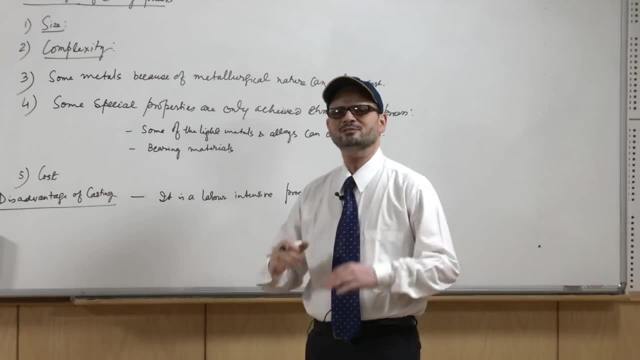 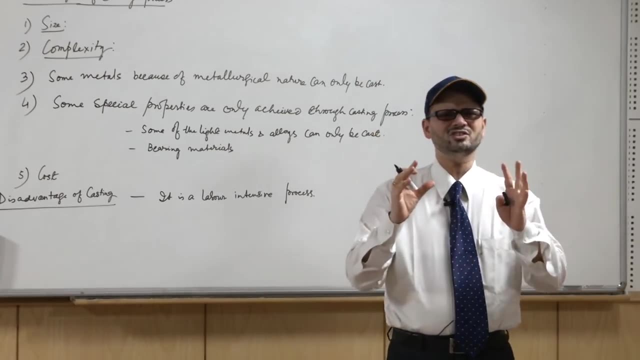 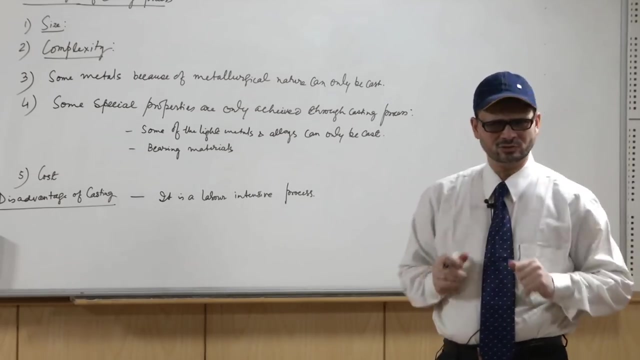 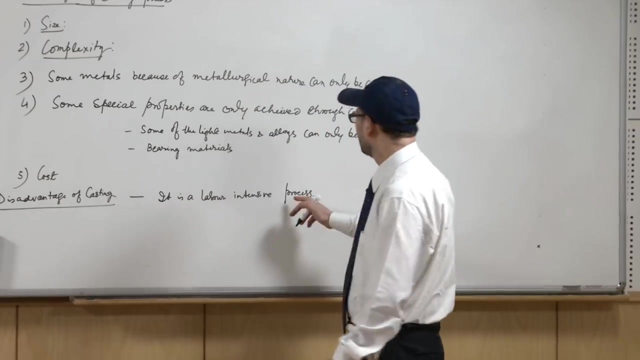 So now even the use of manpower, The use of labour, has been reduced. also, when we talk about having some specialised properties, like you want to have a directional property or the strength in certain particular directions, In that case you will have to go for the further processing of the cast product. then 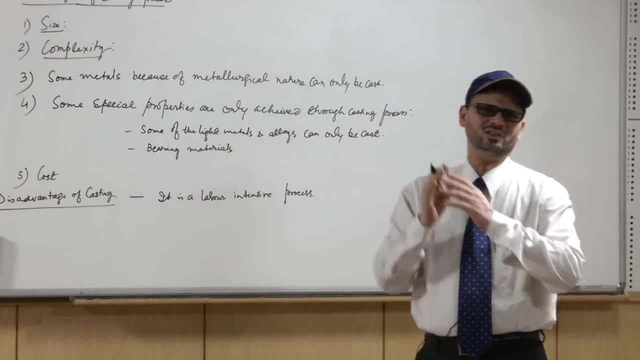 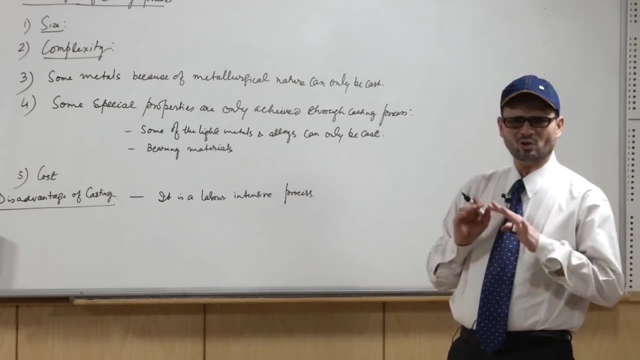 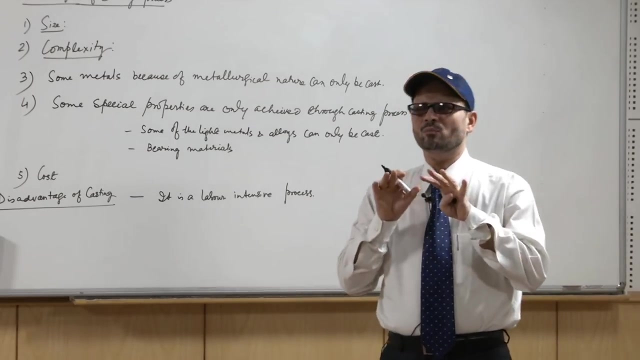 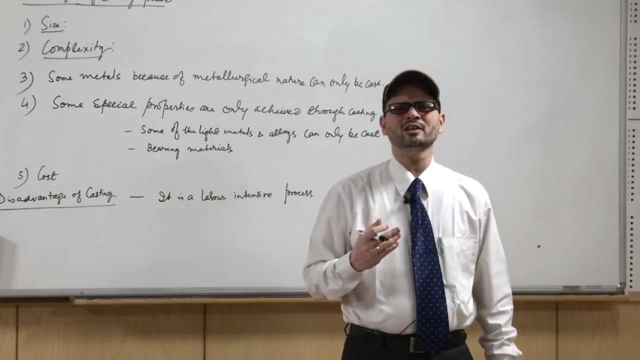 you get like in forging. you get a fibre structure when you are forging under the, under the hammers or the presses, or you are rolling the product to get the product having specialised properties, more strength in certain directions. When we talk about the sand moulding, in that case the finishing also is not completely. 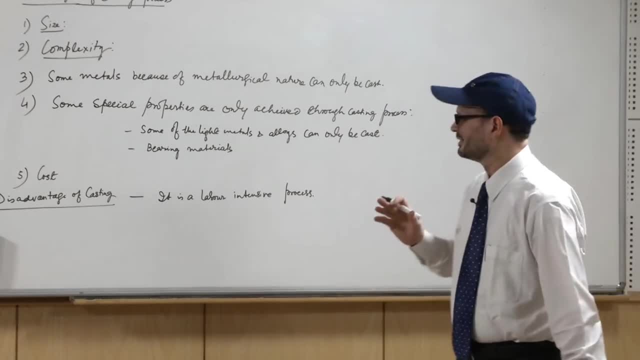 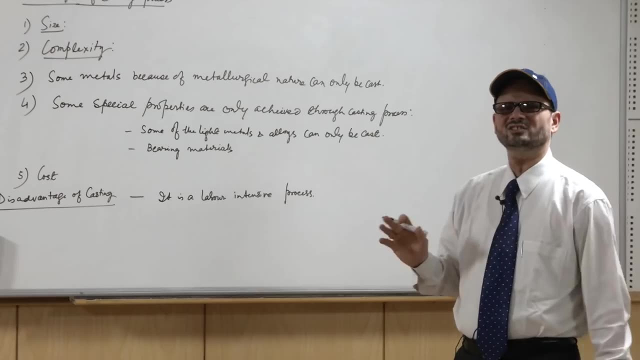 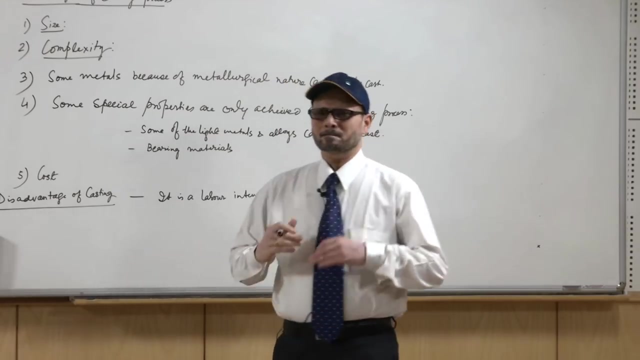 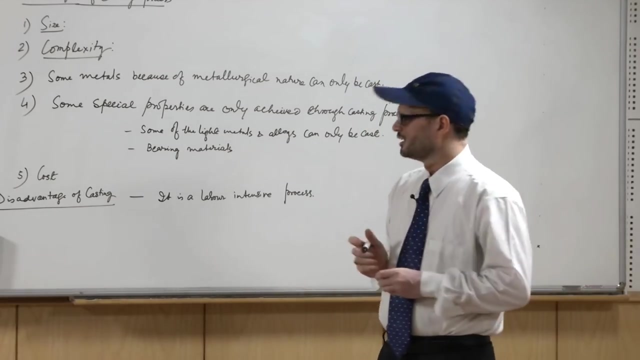 adequate, and in that case you may have to go for the finishing processes. So these are some of the disadvantages of casting process. otherwise there is not many disadvantage and that is why casting is the preferred operation for getting the proper shape of any product. 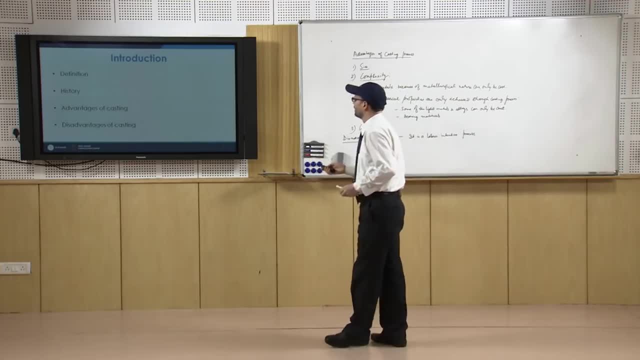 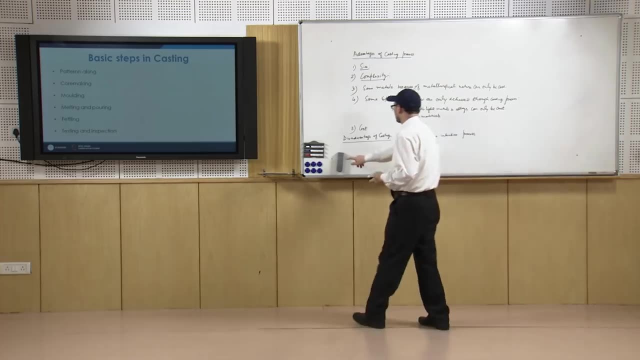 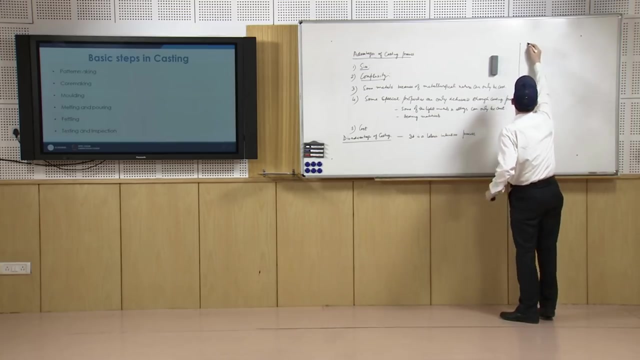 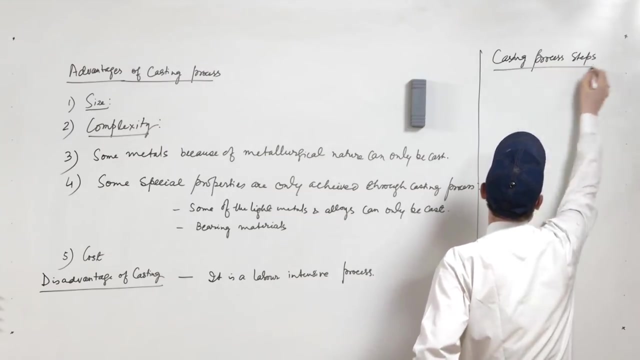 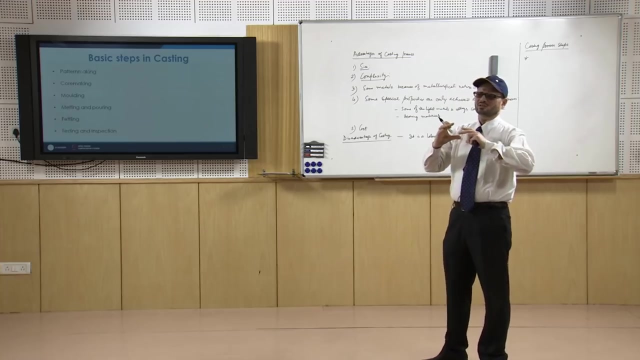 Let us move to next, to the steps of casting. So first thing is technique of casting process. so what is done in a casting process? So, as we discussed, in casting you have a mould in the mould you are wishful making. 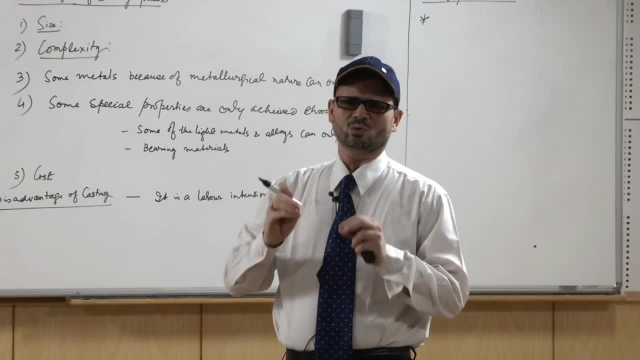 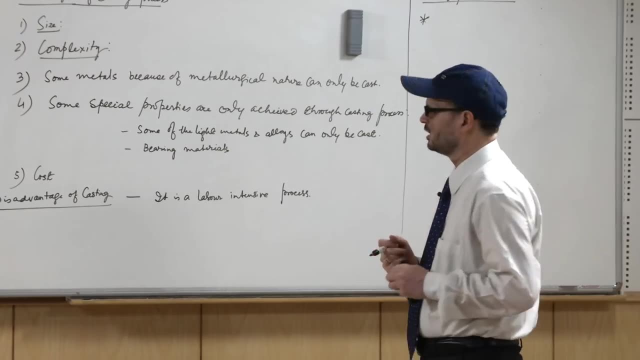 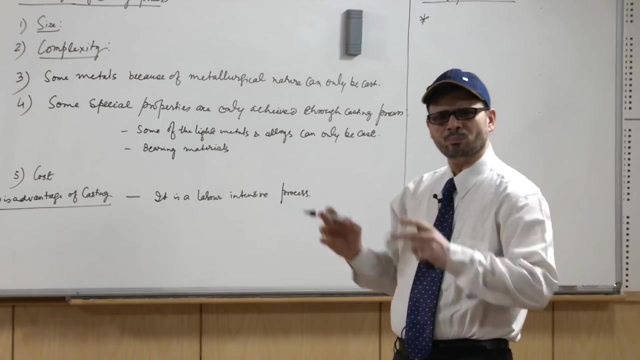 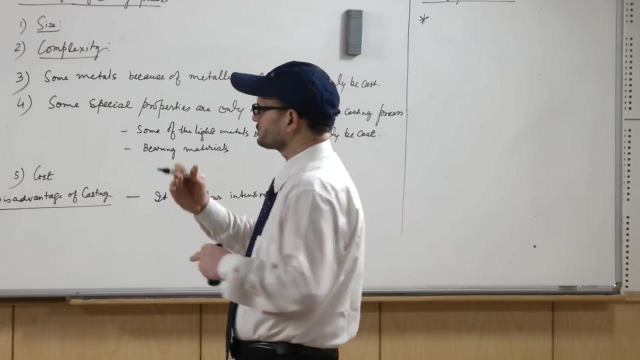 you are pouring the liquid metal which, after getting solidified, has to be removed, and that is your cast product. Now this mold. for this mold, you need the replica of the cast component. So that replica is nothing but a pattern, and this pattern is to be made in a shop that. 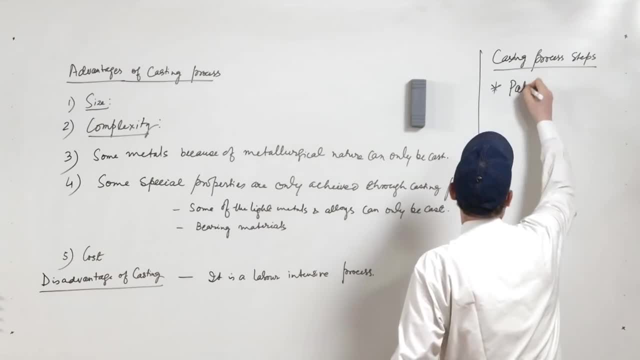 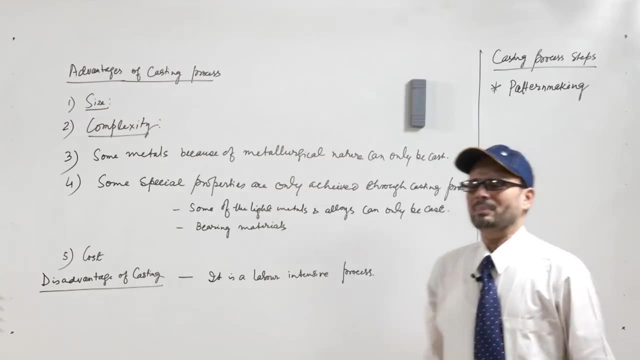 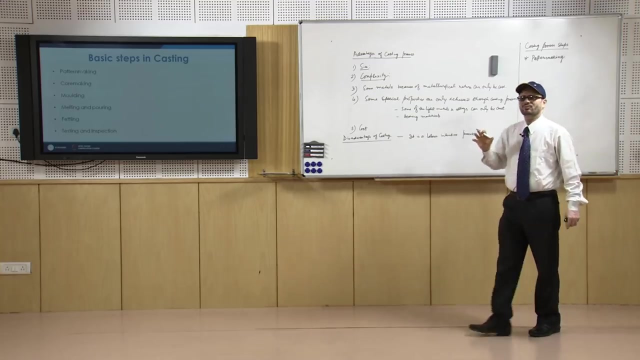 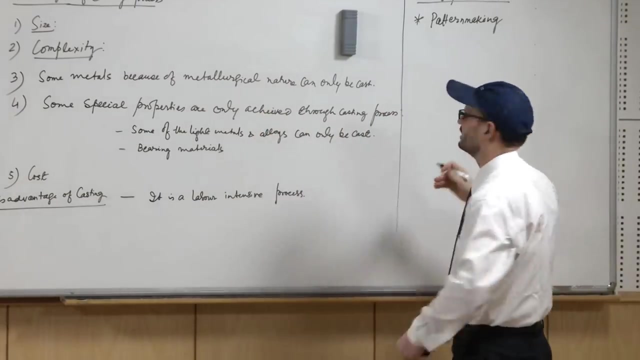 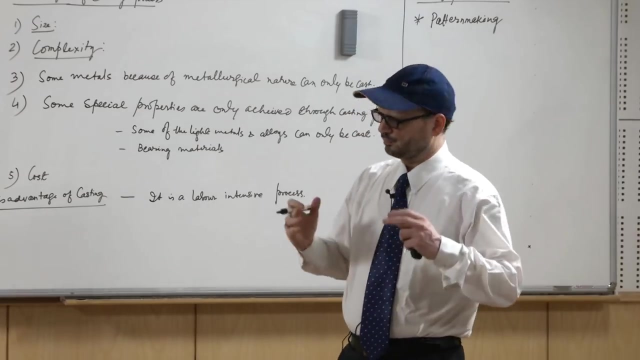 is known as pattern making shop. So first process is pattern making. Pattern making is nothing but making the exact size of the cast product plus certain allowances which we will basically study in the long run. So here this pattern is made of either wood or metal. 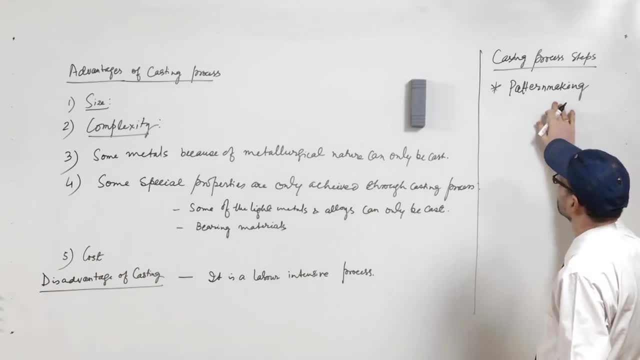 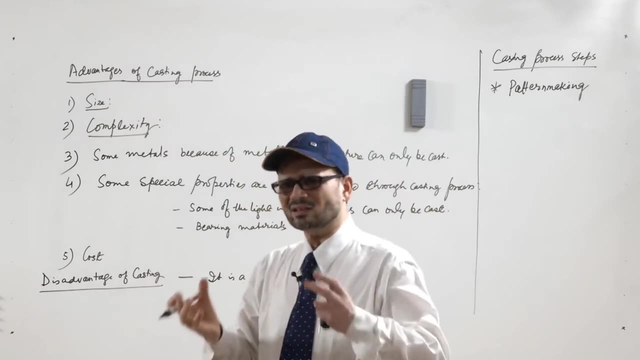 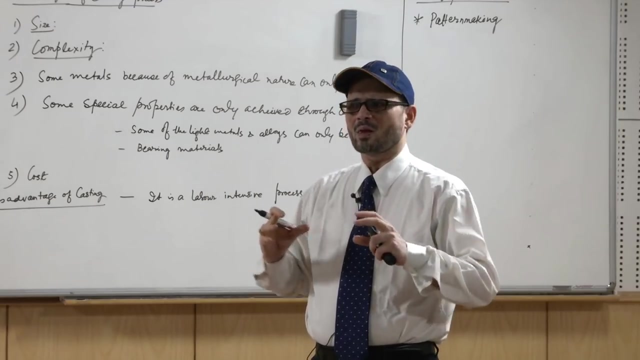 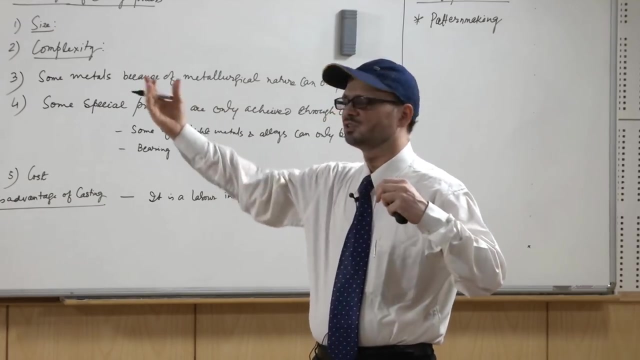 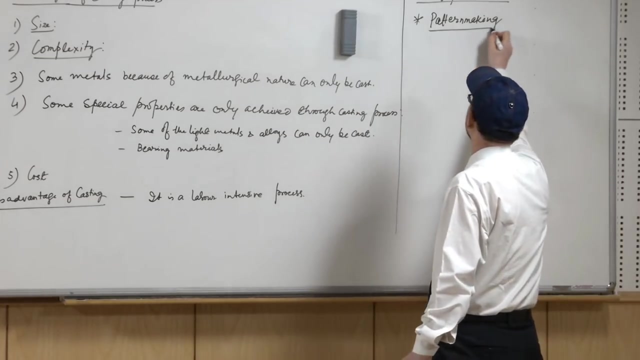 And or even plastic products. nowadays, this pattern making is a separate section which makes this product with this pattern of certain material gives, by considering the allowances. Also, it gives the provisions for supporting the cores, which comes later, for that core prints is there And this is very important because, depending upon the accuracy and the depending upon the 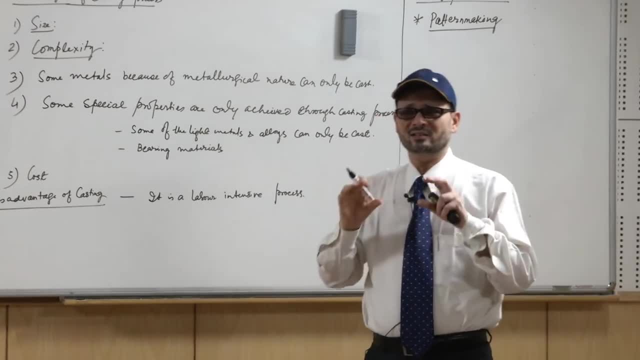 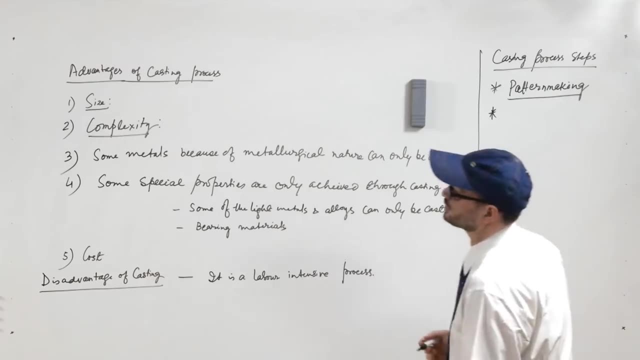 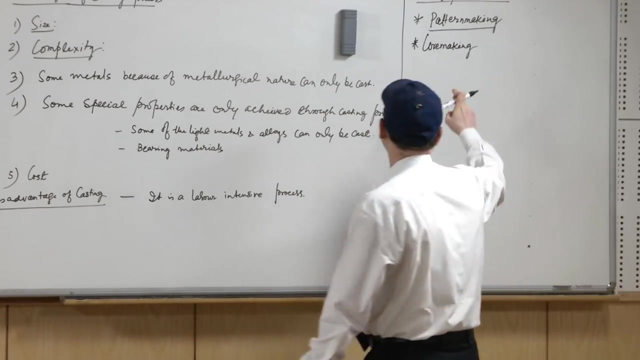 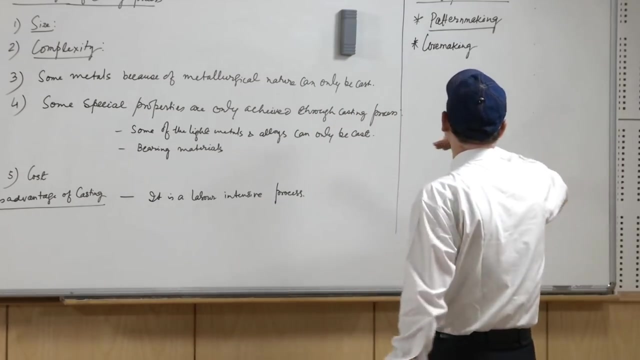 finish of the pattern. You should also expect the quality of cast product. further, there is core making. So when we want to have internal features, certain holes, Or At that time you need to have the core, and this cores are basically made in another unit. 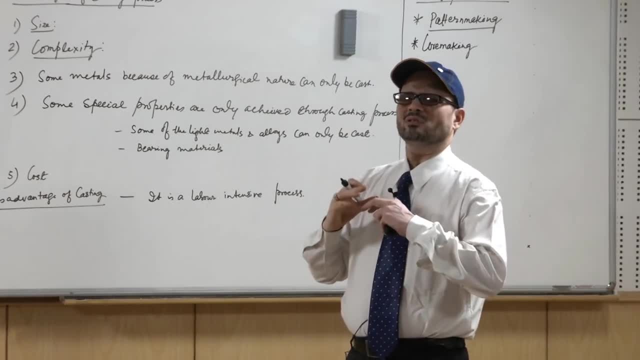 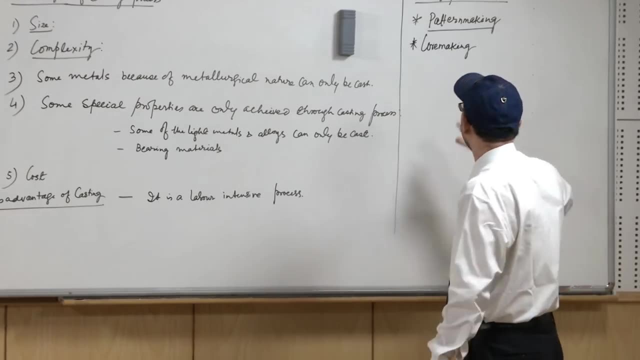 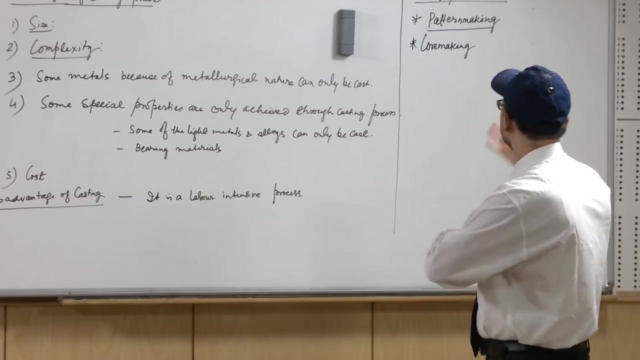 that is core making unit. So cores are normally made of sand, and this is some sand of better purity. Now for this core making you need the core boxes, and for that even pattern making unit is also in tandem, but the core making section is separate. 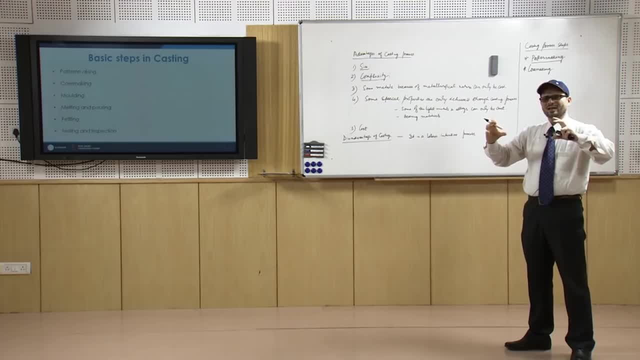 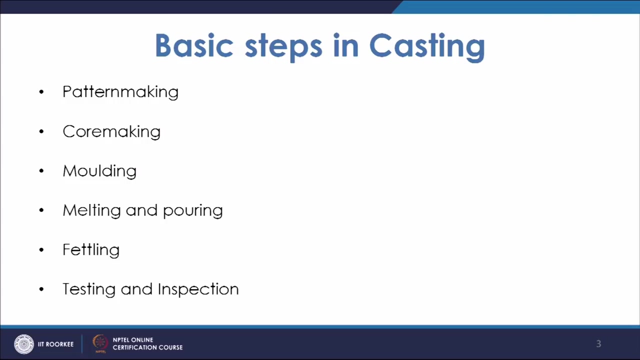 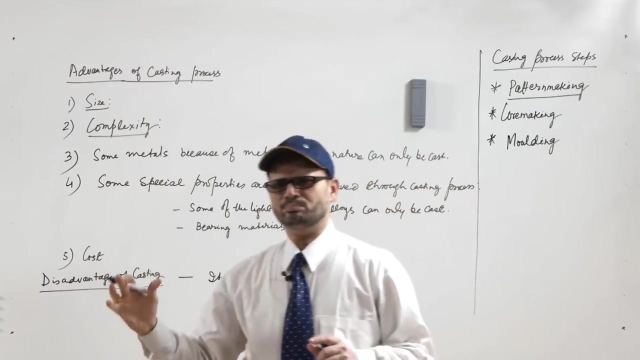 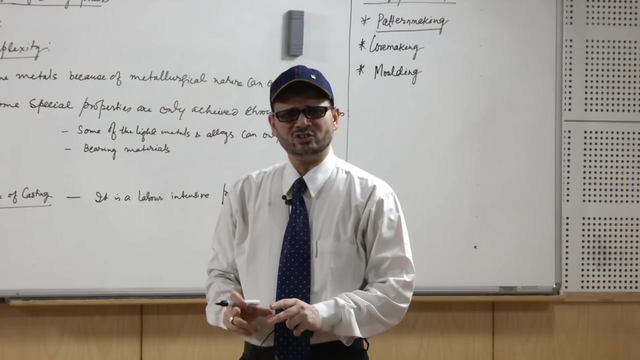 It is responsible for making the cores and keeping the cores in a proper shape and temperature so that it can be used whenever. you have the mold ready and you have to place this core in a in the cavity. Next comes molding. Okay, So you have a molding shop where, basically, you are making the cavity for which the cast 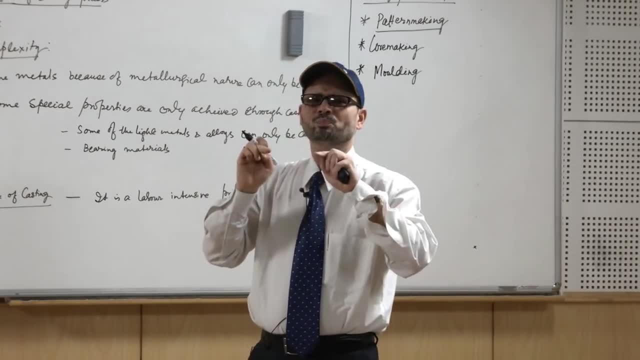 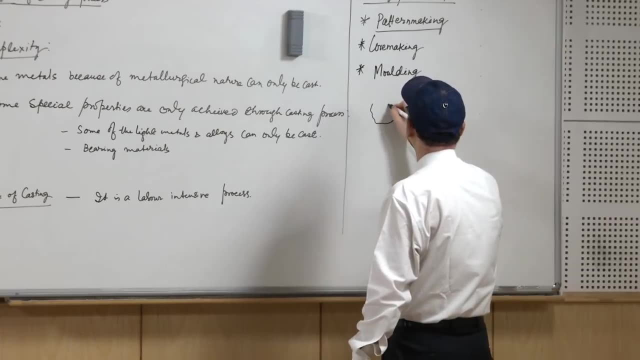 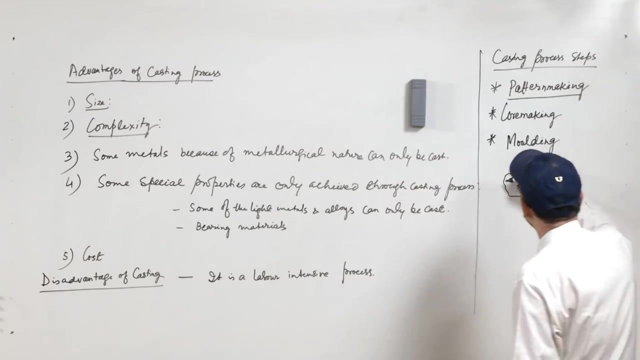 component is required. So basically, you are going to pour the metal in the cavity. So basically, if suppose you have a cavity like this, So ultimately this will be the pattern. Now, what we do is we have to do in such a way that you are putting this molding material 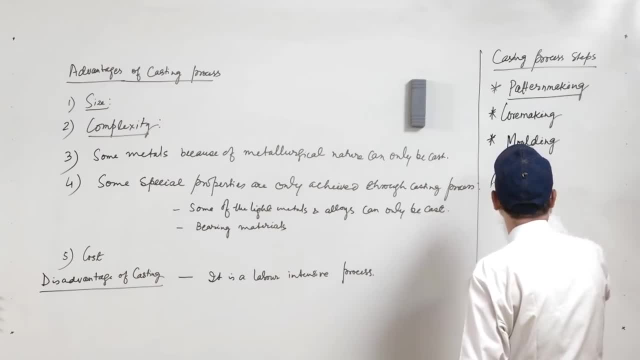 here. So this pattern, Okay, Okay, And this is your molding material. If you talk about the common molding material as sand, we are basically having the pattern in two part and this way, in every part, you are having the molding material packed around. 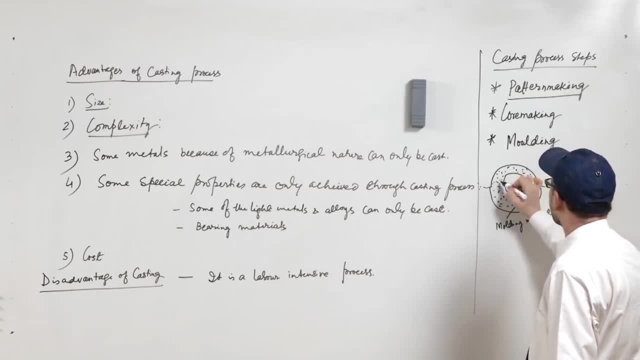 it. Okay, Okay, Okay. So it will be there, but this pattern has to be removed. So, once we remove it, after removing your, this is a hollow part and you have outside. this is the mold. So this hollow part, it is known as cavity. 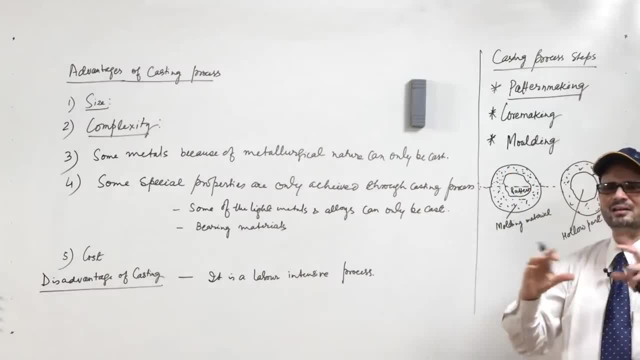 Once we draw this pattern from it, then this becomes a cavity, and this cavity in which the molten metal is to be poured. This molten metal, once it goes here, it will try to lose its heat to the surroundings. H that is heat. 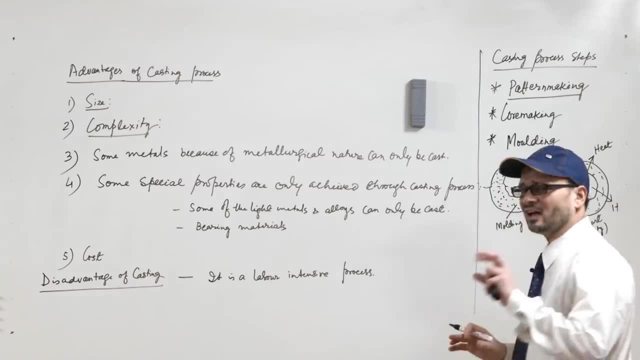 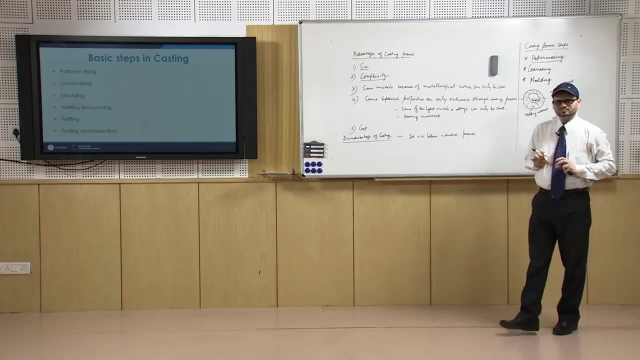 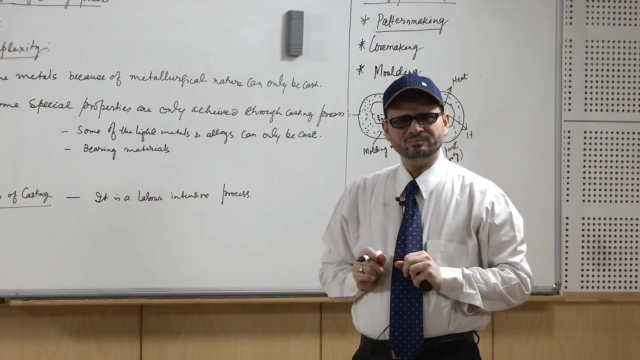 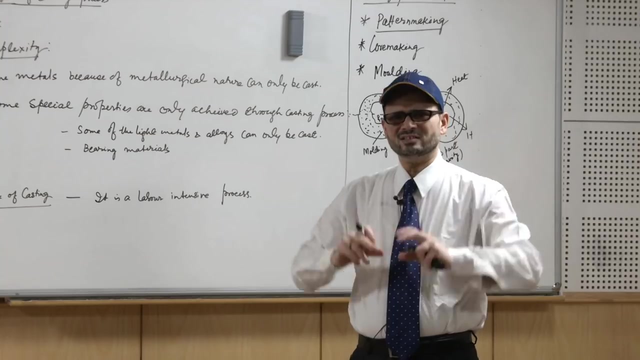 Okay, Okay. So in the molding shop what you have to see is how you have to prepare the mold. The mold has to withstand the weight of the sand by which it is made. The mold has to be shaped in a certain form. for that, it has to be first bring to a state. 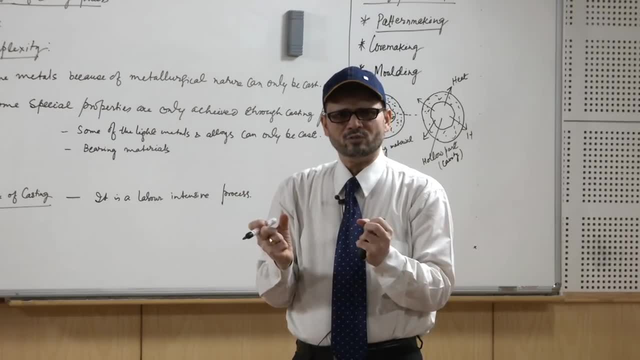 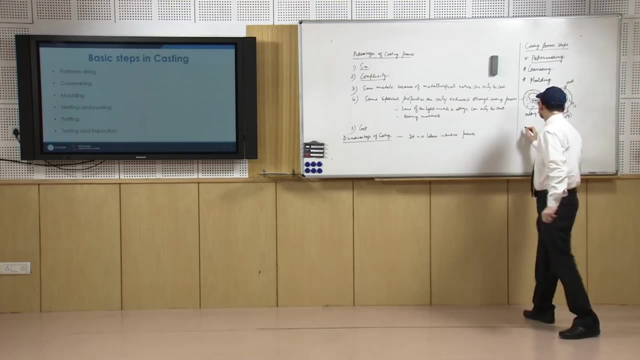 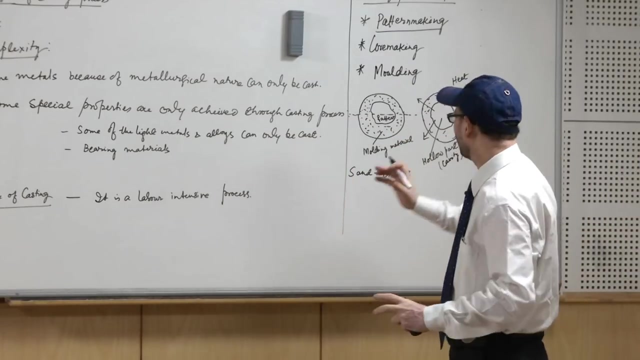 where it can have the cohesion. So for that, basically, in in most of the cases you are putting the binders with the sand. So sand will be used with binders so that it has the cohesive property and you can give any shape to it. 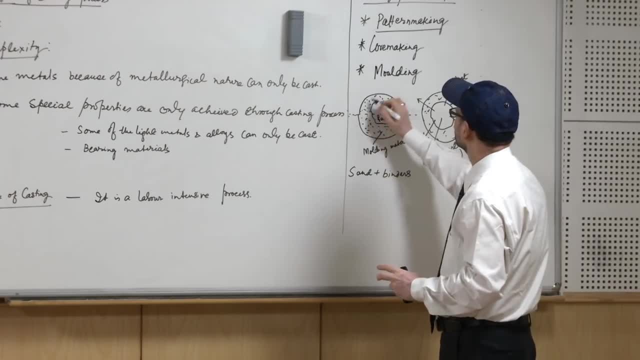 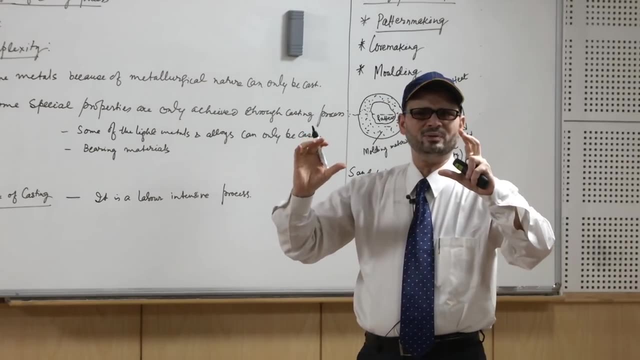 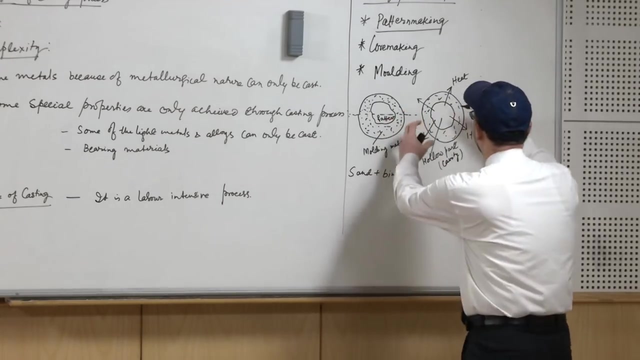 Then this portion is kept around, this pattern. Okay, Okay, Okay, So this is the mold. So the mold is pressed so that it gets a proper shape, with proper strength, and then, with some tool, this pattern is removed and these two boxes are joined together. 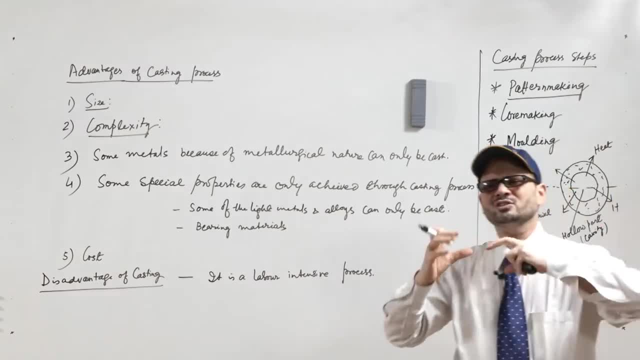 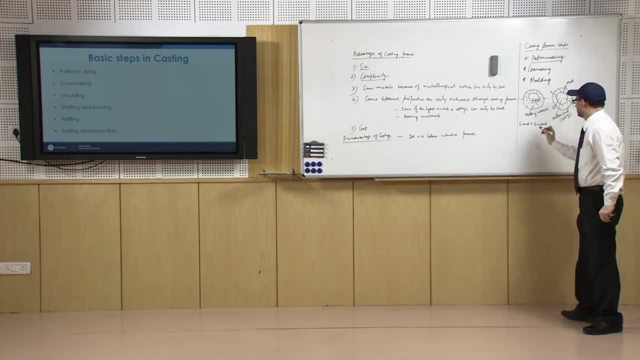 So that you get a cavity and you have the provisions to pour the metal into it. Then you are pouring the metal. You also add additives that we will discuss later. What are the additives? What are the additives? Okay, What are the functions of the binders and additives? 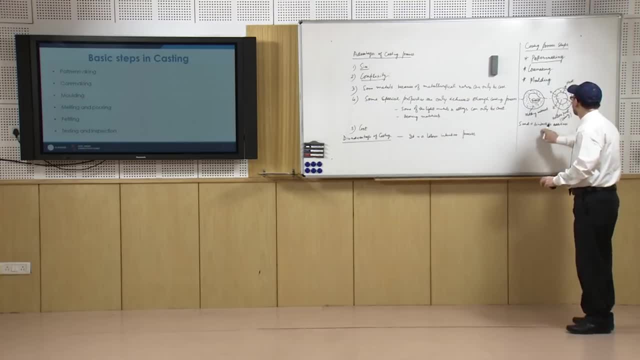 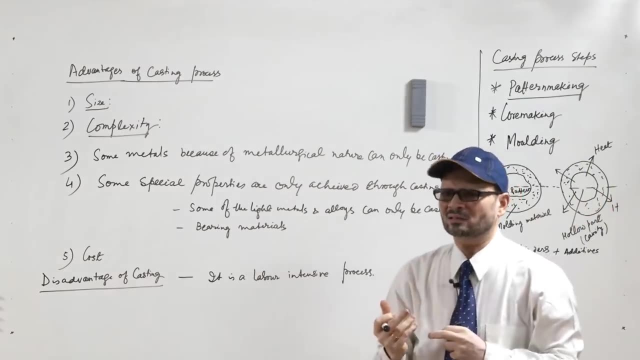 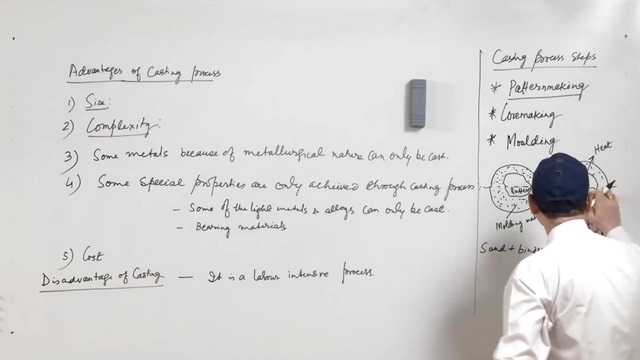 So basically we are putting all that so that it has a flowable property. It goes around the pattern and takes all the minute. you know details. and then this, basically, once you have this shape, in that when the metal is poured it gives you the cast product. 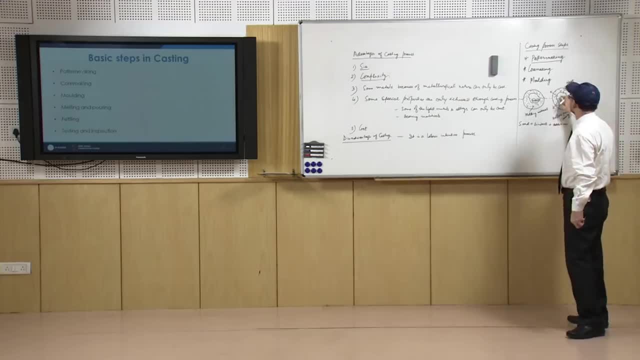 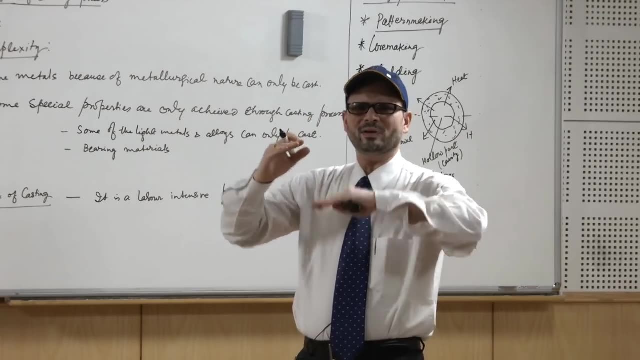 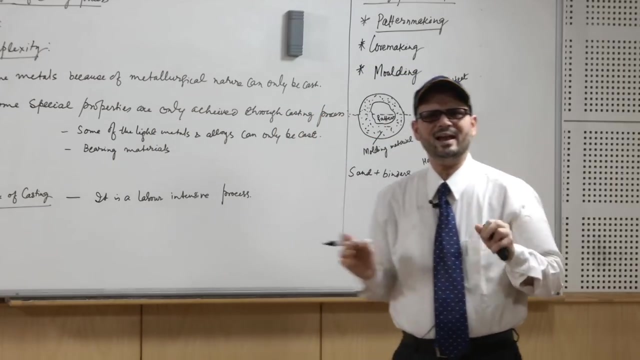 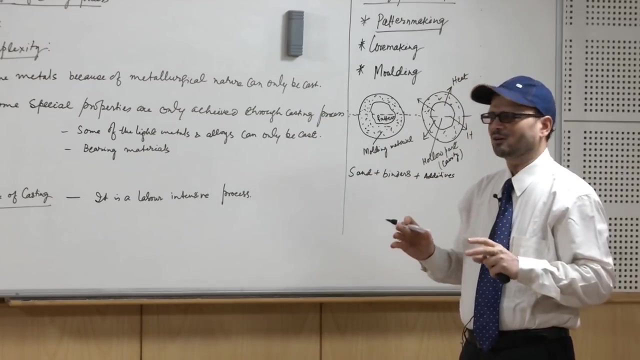 after solidification. So in the molding section you have different kinds of molding boxes. You have bottom, top and middle molding boxes. You have different units for basically mixing of sand. You have units for the baking of sand, baking of the mold, and once that is ready, then when? 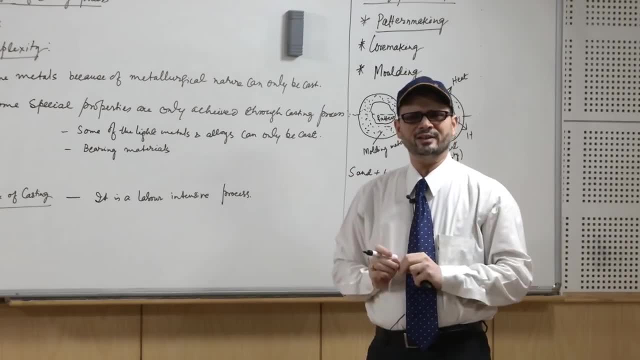 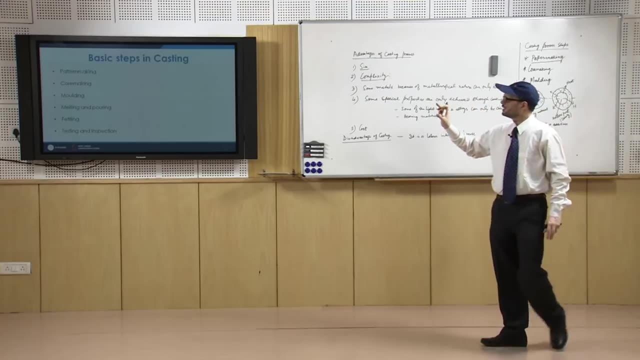 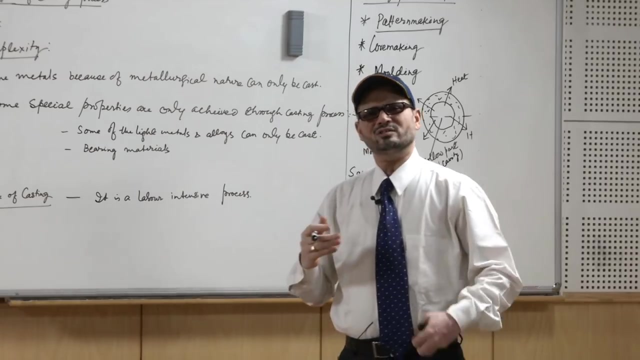 the pattern is removed. Okay, Once you have baked the unit, your mold is ready for the pouring part. So that way, molding section is important. you have to prepare the mold. The mold may be of sand or, if you are- we are talking about the permanent molds- we may. 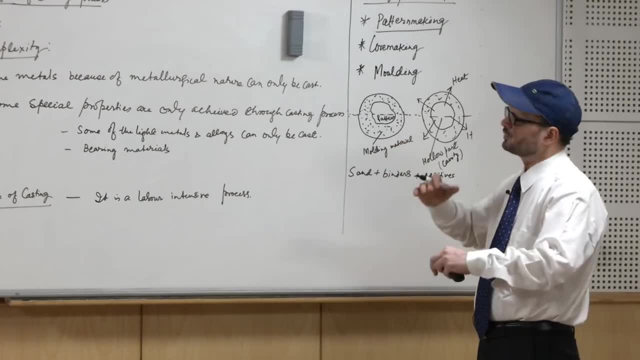 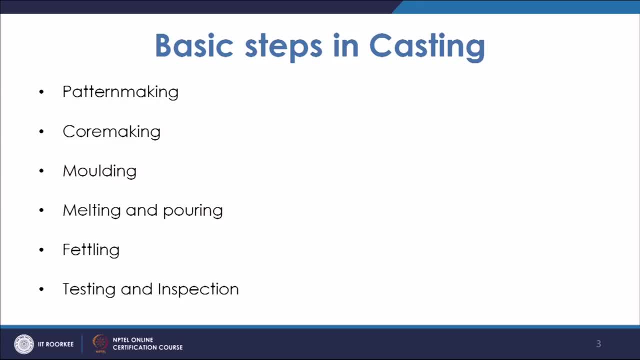 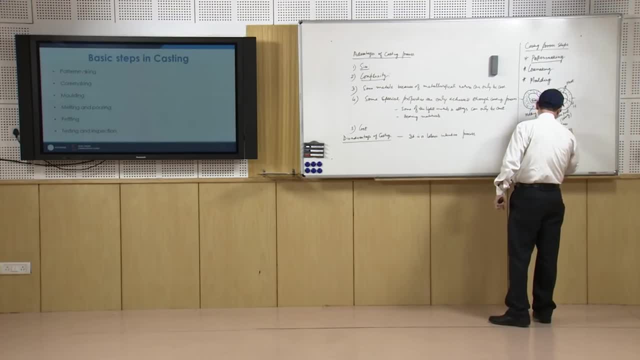 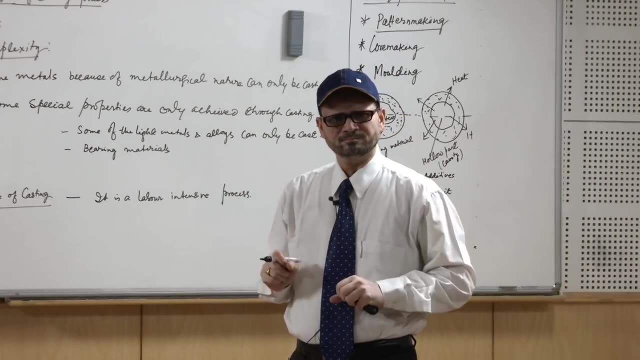 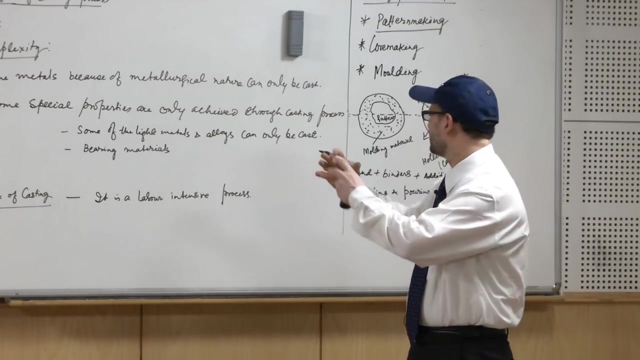 So before finding the mold, we have to prepare the mold. Now let us get down to the components of the mold. First, we need to get the mold in contact with the material found, understood, wise, then we can build the mold. 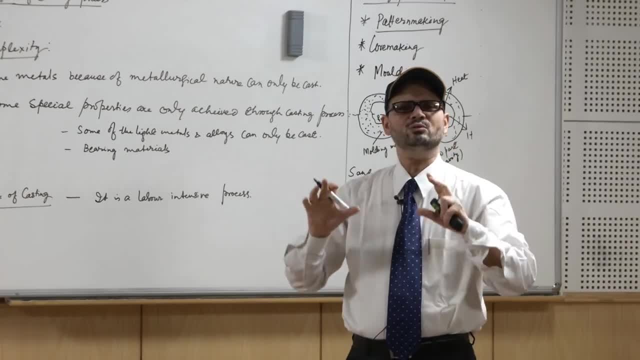 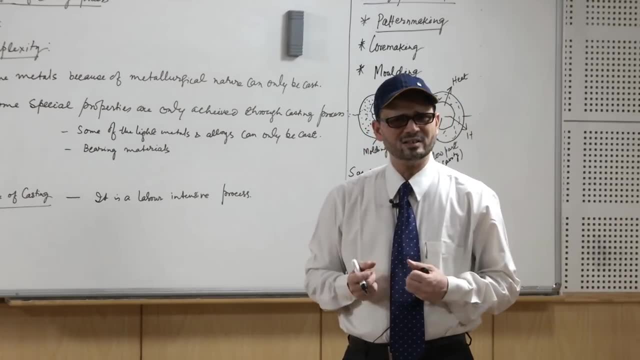 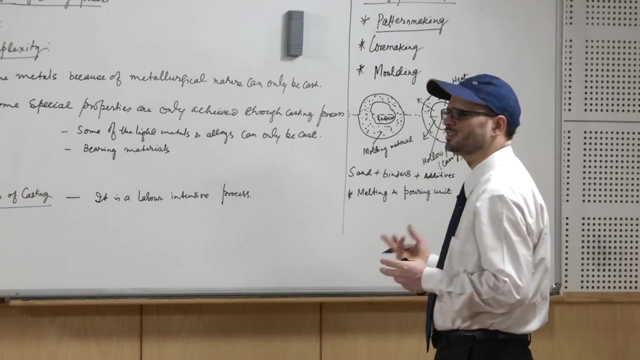 transported to the place where the molding has to take place. so the furnaces may be of different type depending upon the need of requirement or requirement of the amount of metal to be melted and to be poured. so you may have the furnaces like cupola furnace. 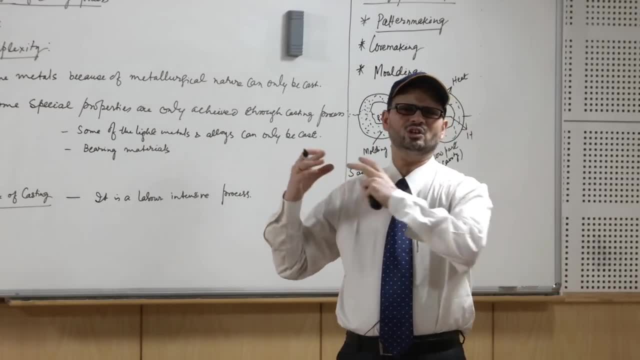 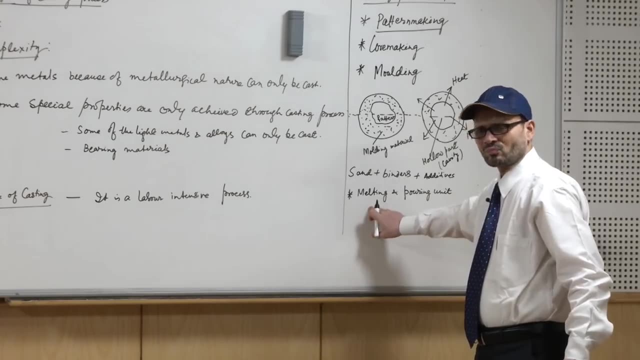 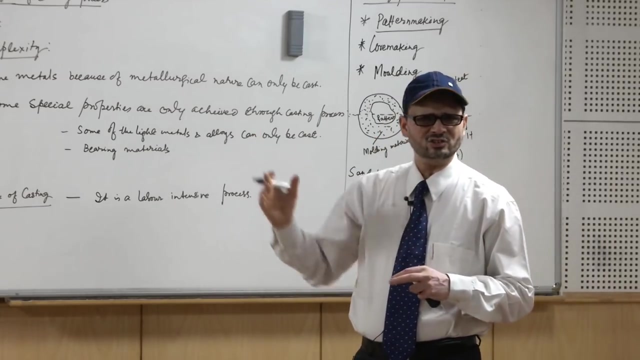 for cast iron. you may have the arc furnace, you may have the induction furnace. so all these furnaces are placed in the melting unit you have. from there, you will have to transport these metals through cranes or by other means, and then you have to bring it. 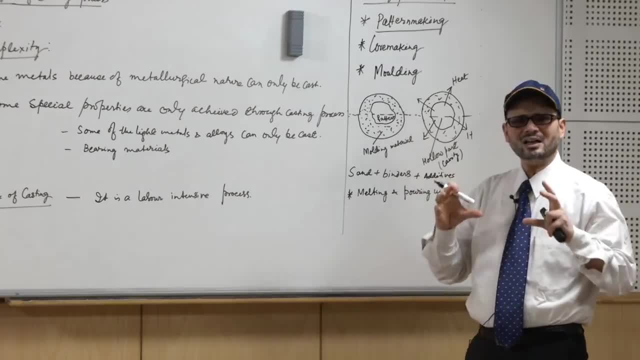 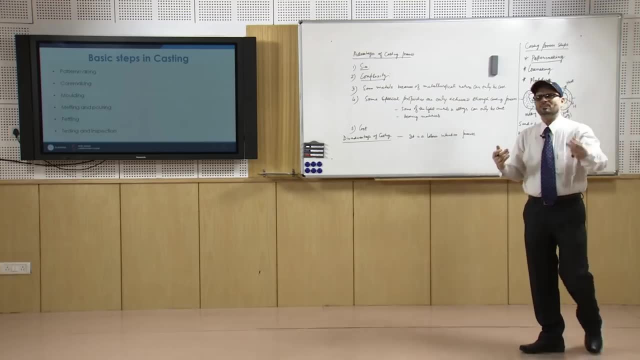 to the place where you have to cast it. so sometimes if the mold is the smaller, it can be transported to other place, but if the mold is heavier, basically in the molding unit itself the metal is to be transported and there it is to be cast. 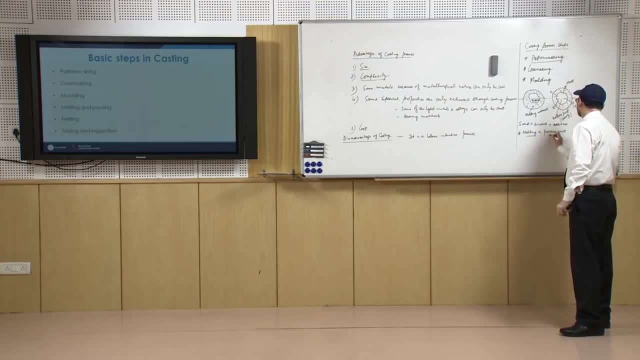 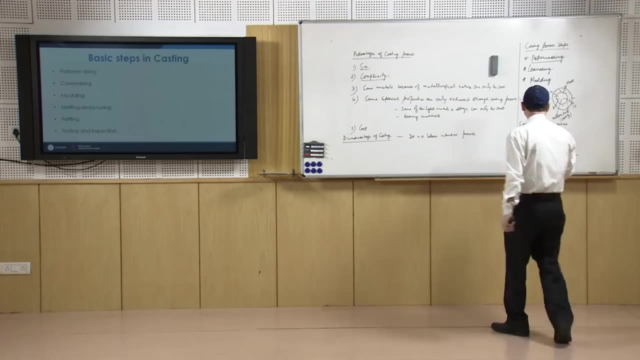 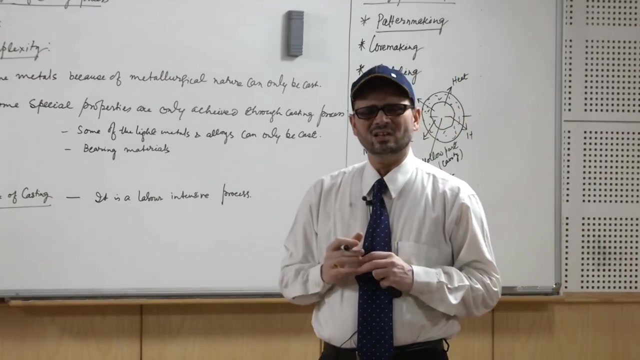 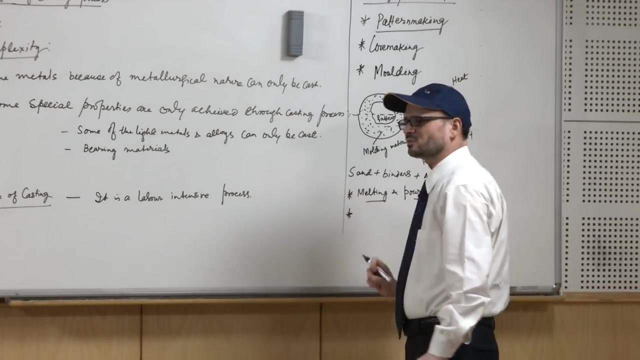 So this is how this melting and pouring unit serves the purpose of making the cast product. Now, once you have poured the material into a mold, as we have already discussed, this material undergoes solidification. Now, once the material is solidified, it has to be taken out. 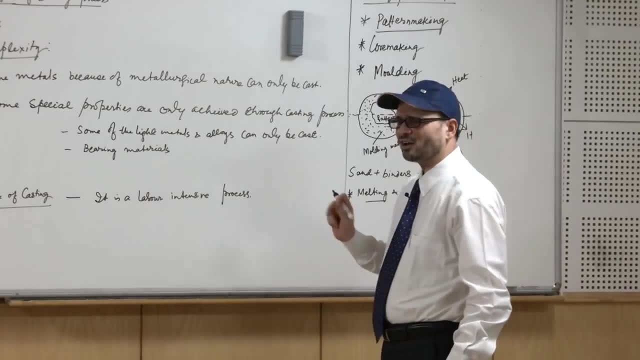 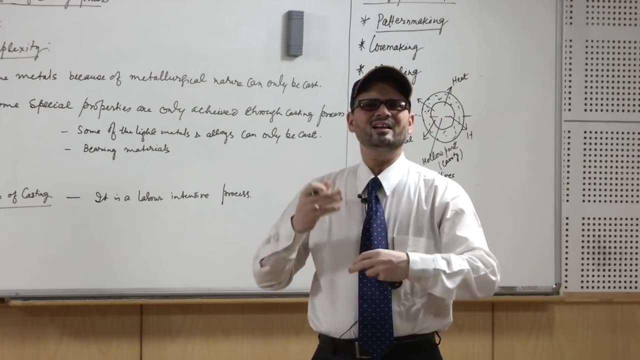 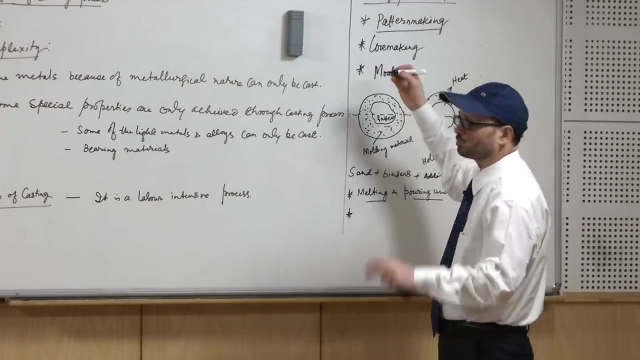 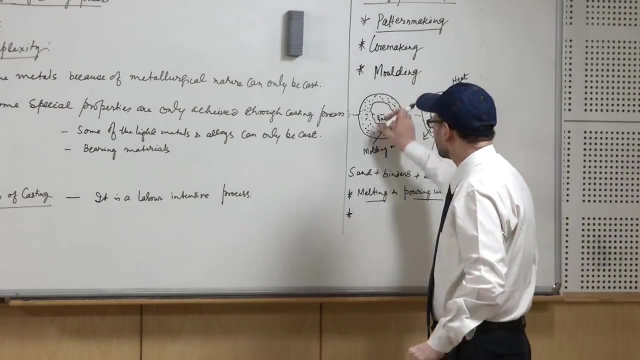 Now this material or this product, this cast product has a lot of other sections, which is out other than the original cast casting. So you may have a mechanism for pouring the material through a funnel shaped mold, So you may have a attachment, or you may have a horizontal way to pass the liquid metal. 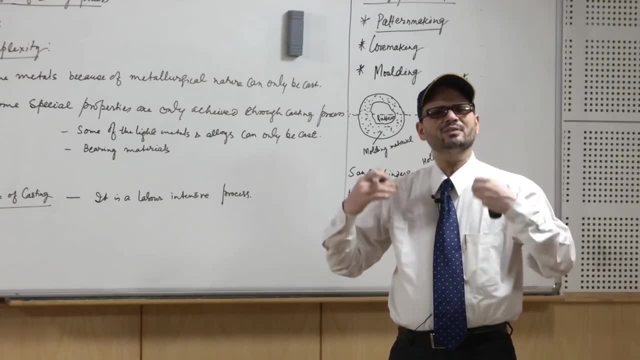 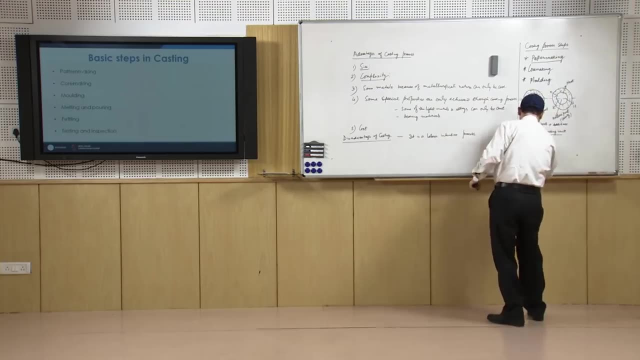 or you may have a riser which takes into account of the shrinkage. all these are to be removed, So that is done through the process of fettling. So fettling is nothing but removing all the unwanted material. So this is how it is done. 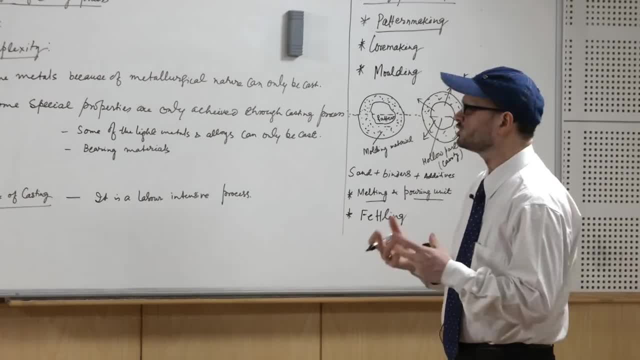 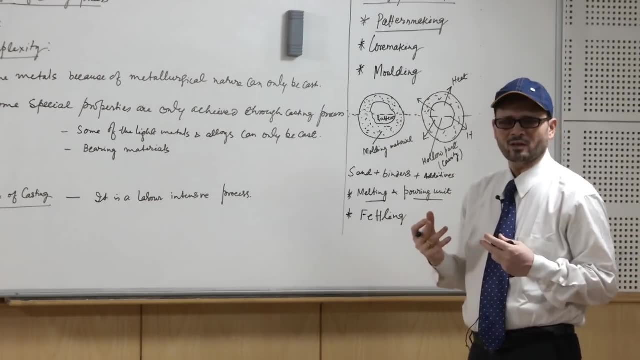 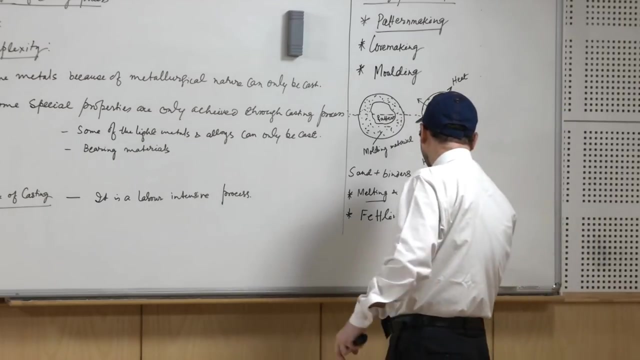 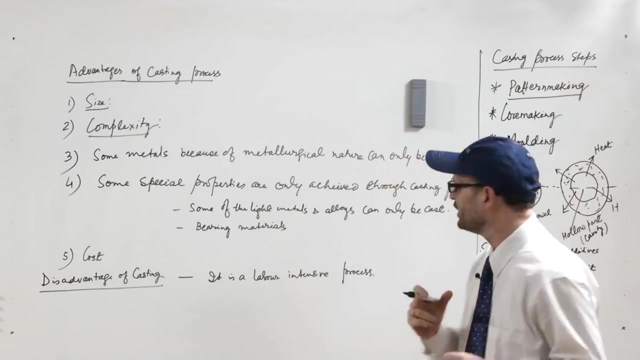 So if you have unwanted attachments or the portions which are attached to the cast product, you have to basically also clean the unburnt sand, you have to clean the scale. all these fettling and cleaning. these are done so that you have to further use this material. 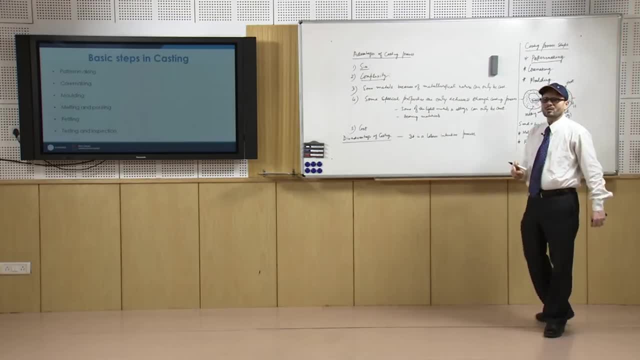 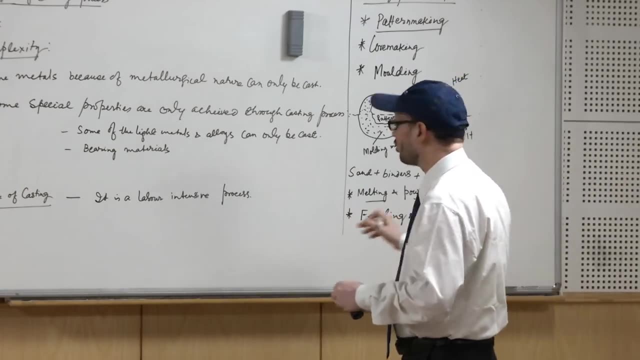 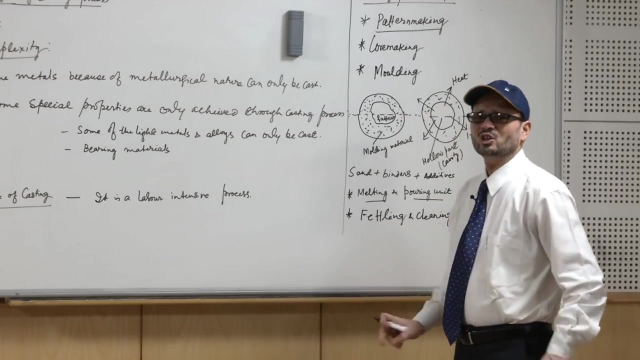 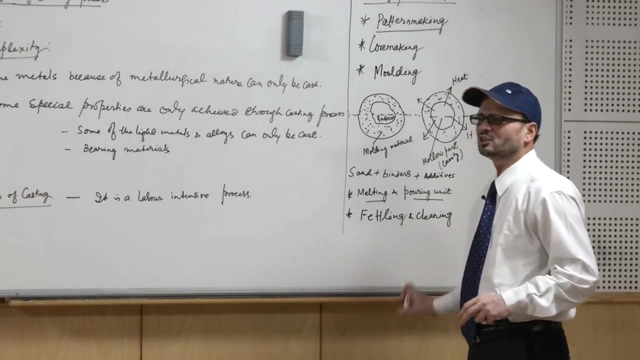 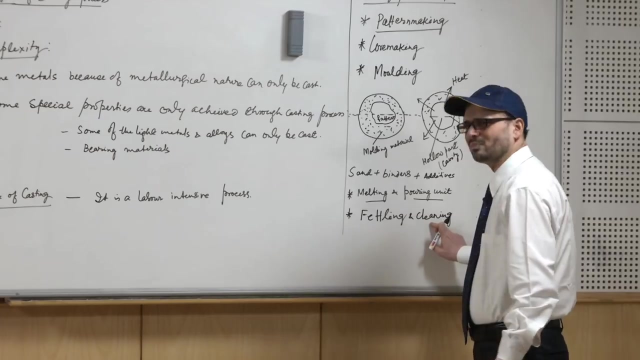 So in this case you have the provisions For either breaking the extra attachment or you may go for cutting these attachments by flames or by electric torches. For cleaning you may use the liquid solvent based agents or you may use solid particles of iron shots- they also are used, so that is, by shot blasting. 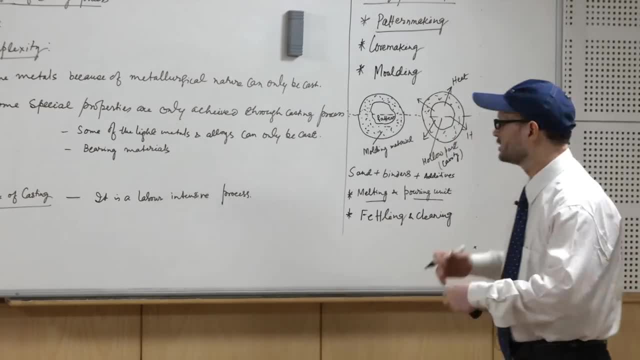 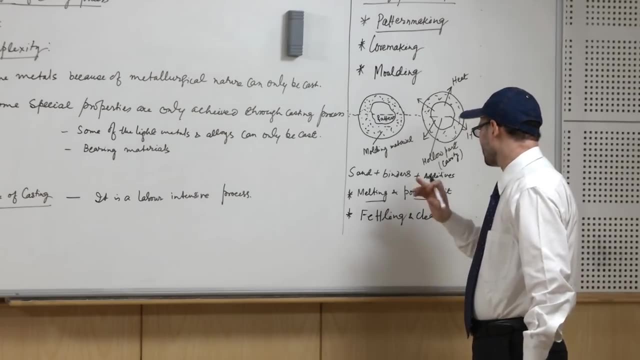 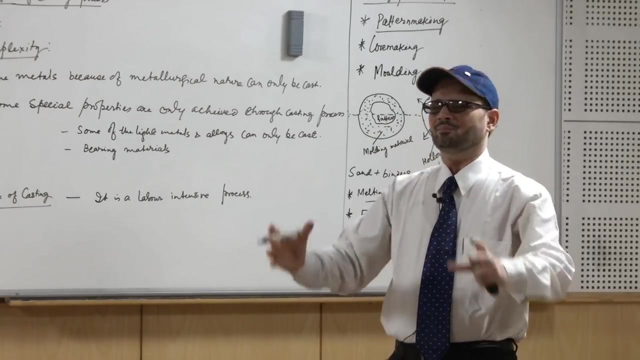 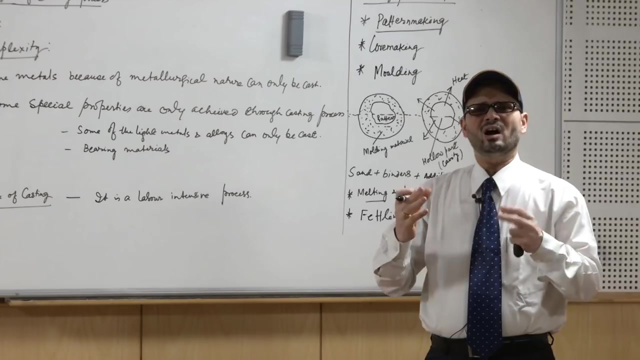 You may use sand also. So this we will discuss when we will talk about the fettling and cleaning in the towards the end of the course, and the purpose is to give the material a final finish or final look how the metal has to be shown, how its surface roughness is, how you have to go adn. 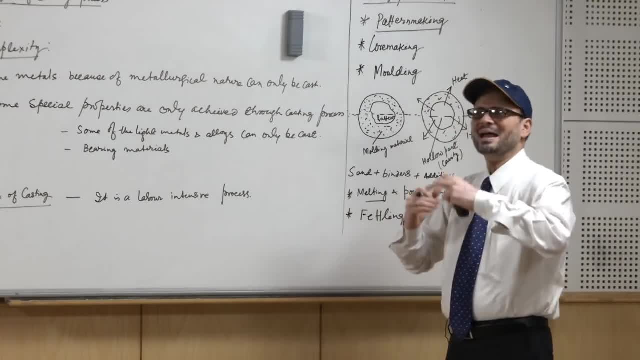 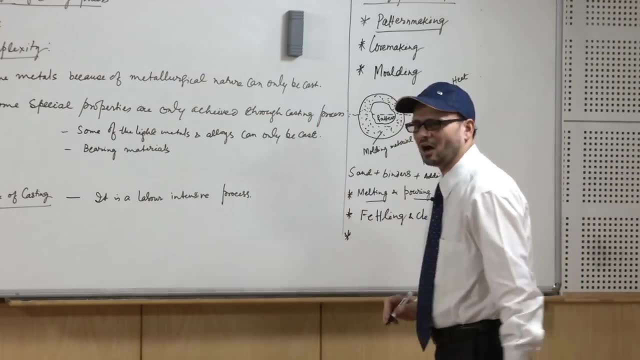 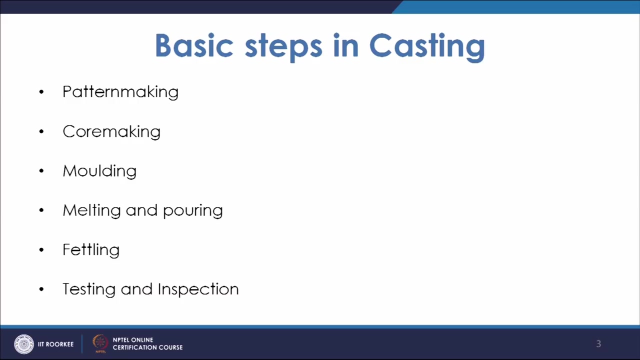 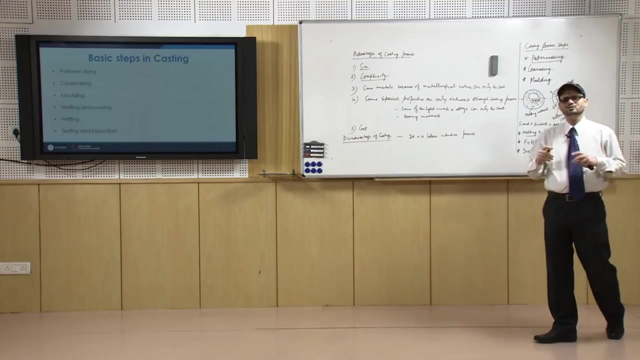 you have to change, Ok, basically pack it and you have to supply it to the customer. before that, however, you will have to go for inspection and testing. so, finally, once you have cleaned the product and you the product is ready, you will have to also ensure that the product is metallurgically. 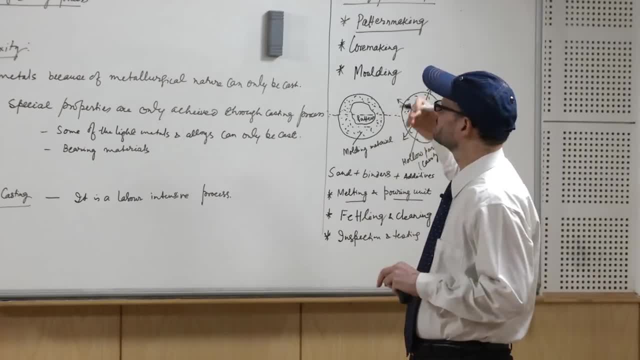 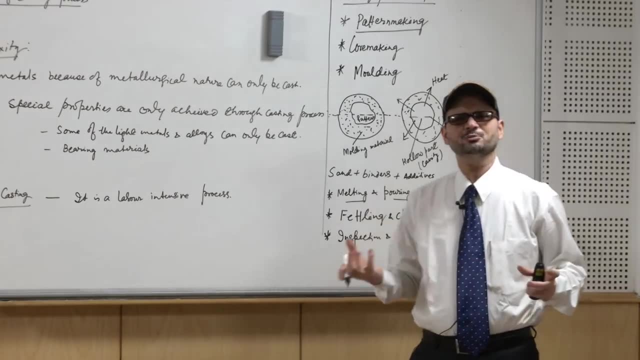 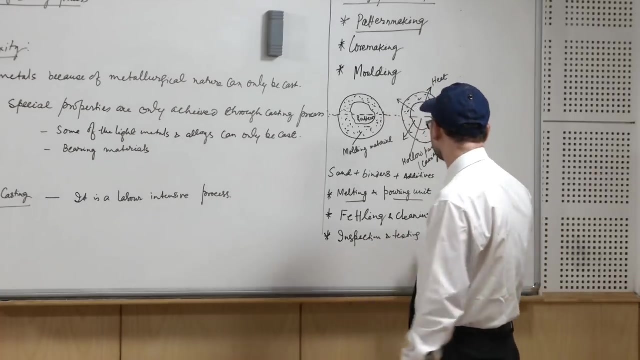 ok, it does not have defects, as we will discuss about these defects in our in the long run- but a cast product because its a phase change process, you have the possibility of having different type of defects. the defects may be on the surface, it may be inside it, so there,